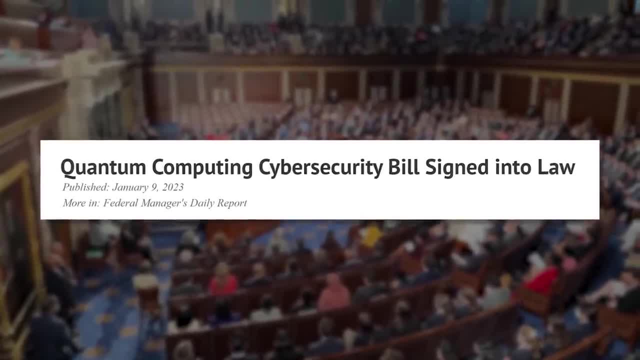 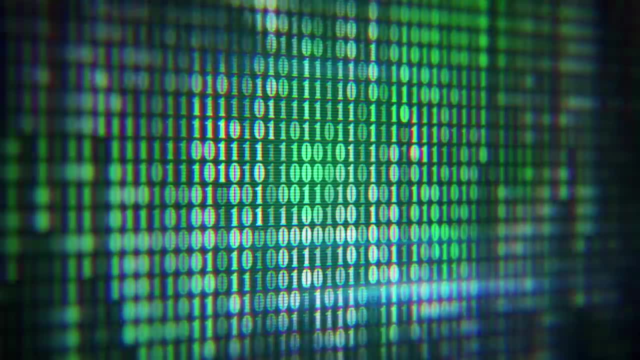 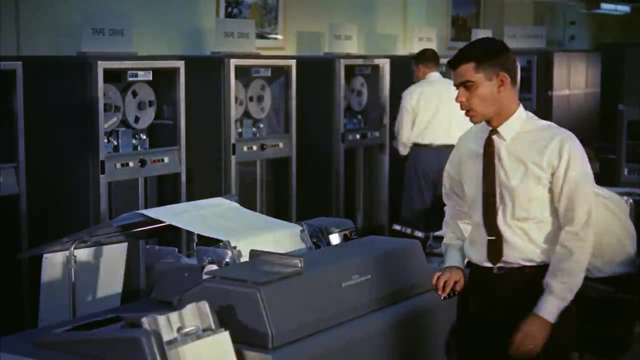 passed legislation mandating all agencies start transitioning right now to new methods of cryptography that can't be broken by quantum computers. Our current encryption schemes have been remarkably successful, working effectively for over 40 years. Up until the 1970s, if you wanted to exchange private information with someone. 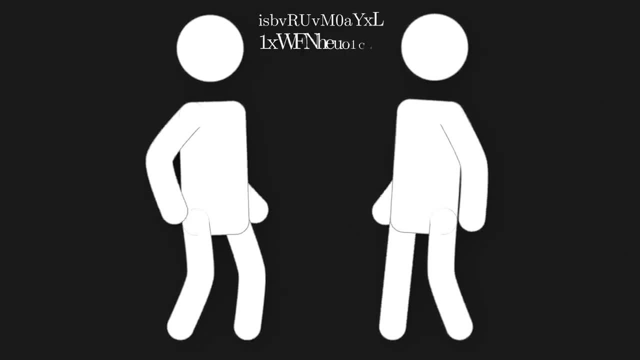 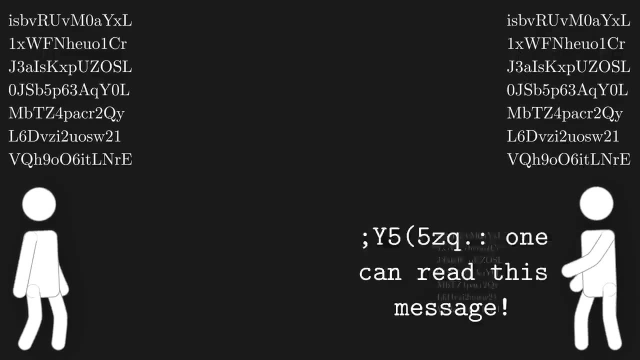 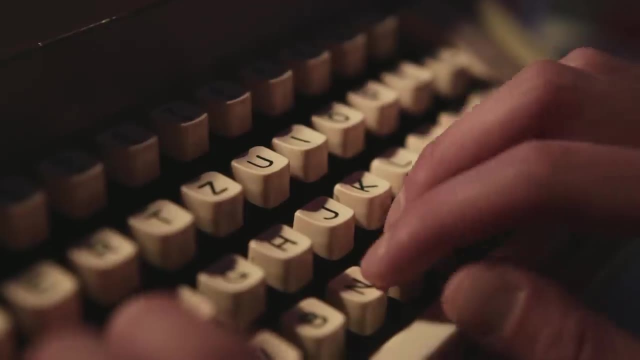 you would first have to meet up in person and share a secret key. This same key would be used to encrypt and decrypt messages, so it's known as a symmetric key algorithm. As long as no one else gets their hands on the key, your messages are safe. But now what if you want to send? 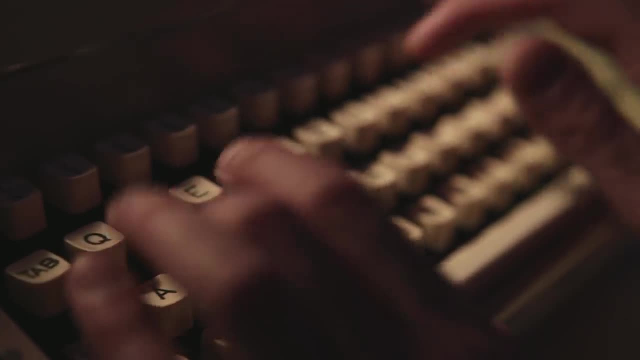 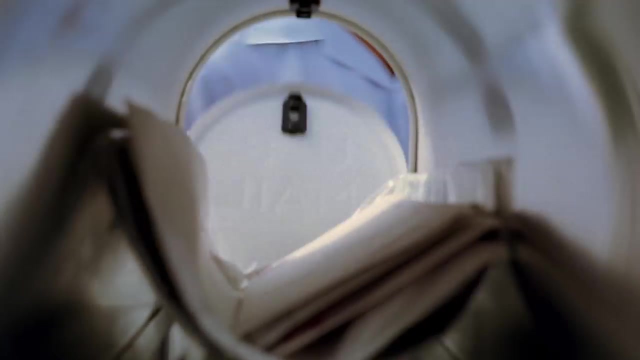 information to someone you've never met, and it's too hard to arrange an in-person meeting. You can't share a key over an unsecure channel like a phone line or the mail, because it could be intercepted. And this is what, in 1977, led three scientists. 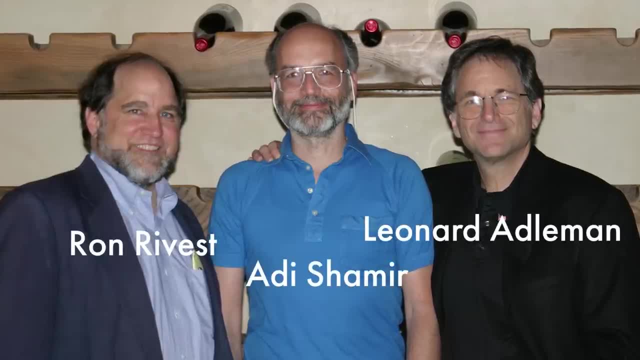 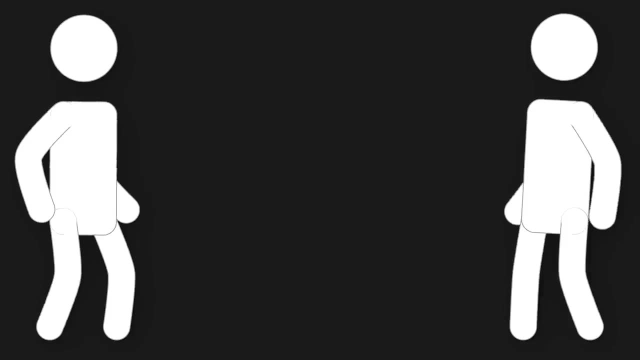 Rivest, Shamir and Adleman to come up with an encryption breakthrough. Today it's known by their initials, RSA, And it works something like this: Every person has two really big prime numbers all their own, which they keep secret. They multiply these numbers. 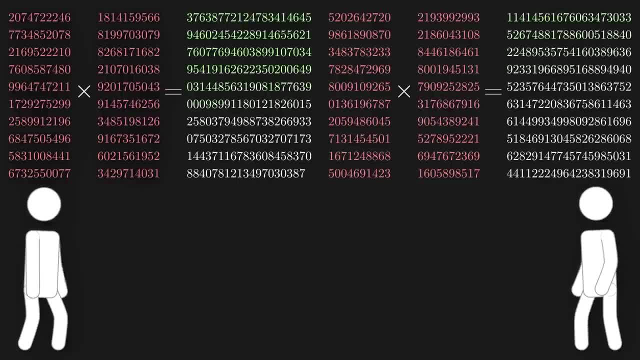 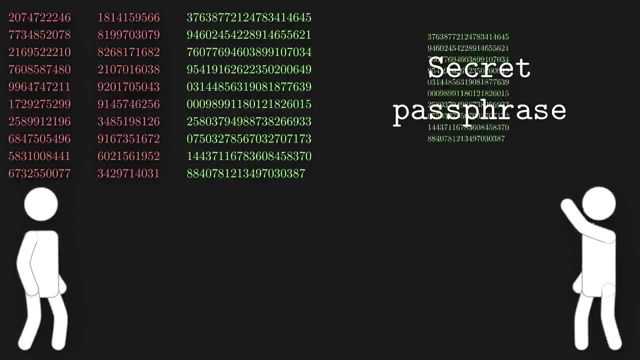 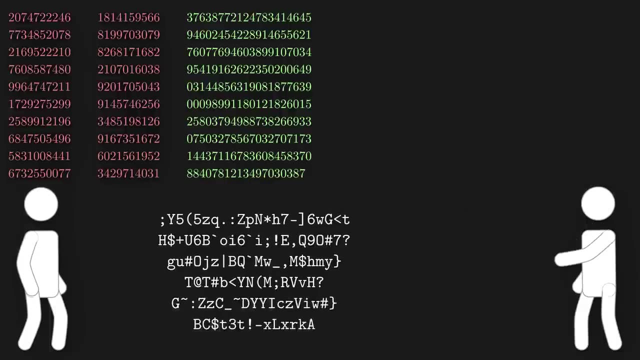 together to get an even bigger number which they make public for everyone to see. Now, if I want to send someone a private message, I use their big public number to garble my message, and I garble it in such a way that it is impossible to un-garble without knowing. 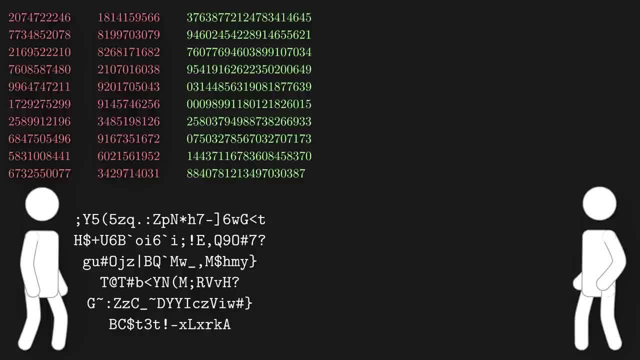 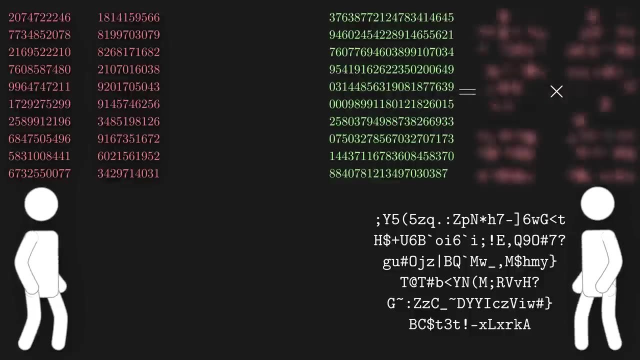 the two prime factors that made that number. This is an asymmetric key system, since different keys are used to encrypt and decrypt the message, So it's easy for my intended to decode, but impossible for everyone else, unless they can factor that large public number. 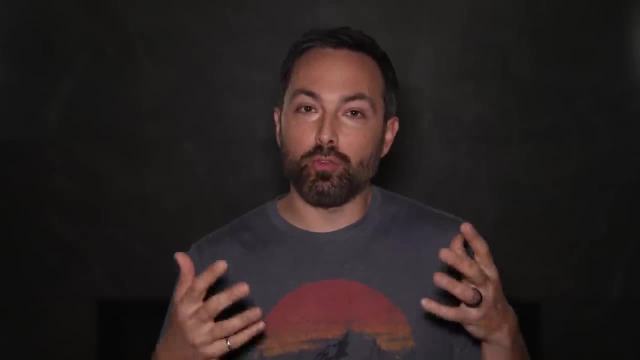 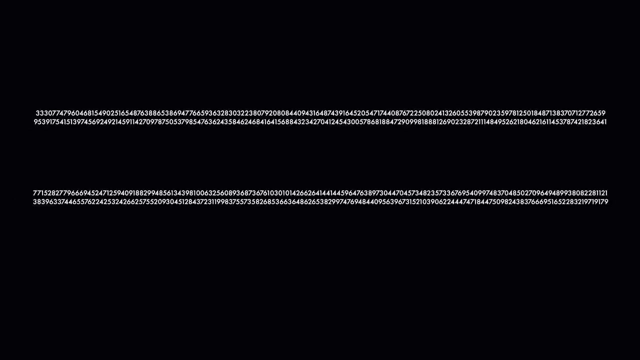 Now someone could try to factor it using a supercomputer in the best known factoring algorithm, the general number field sieve. But modern cryptography uses prime numbers that are around 313 digits long. Factoring a product of two primes this big even with a supercomputer. 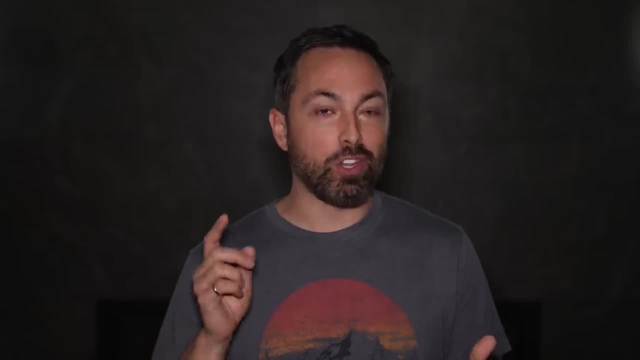 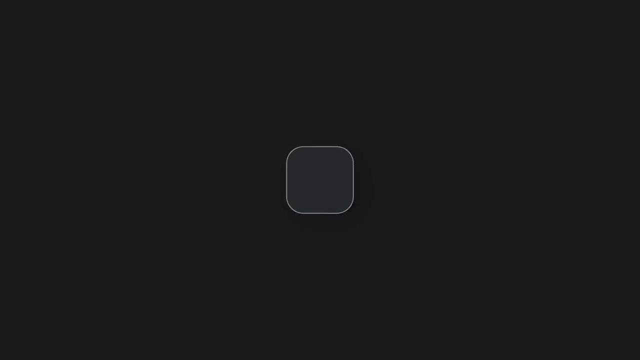 would take around 16 million years. But not on a quantum computer. See, in normal computers a bit can only be in one state at a time, Either a 0 or a 1. So if you had two bits, they could be in one of four possible states. 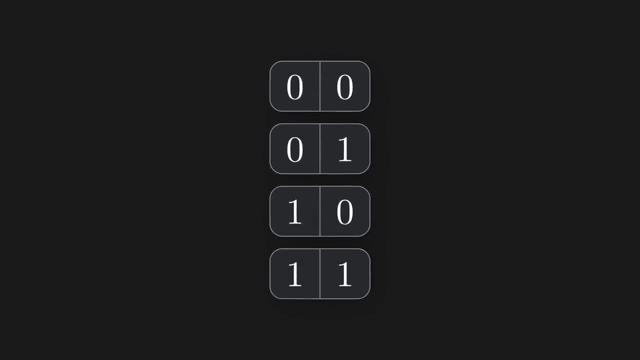 0, 0, 0, 1,, 1, 0, or 1, 1.. Let's say, each of these states represents a number: 0,, 1,, 2, or 3.. If we want to do a calculation, for example raising 7 to the power of one of these numbers, 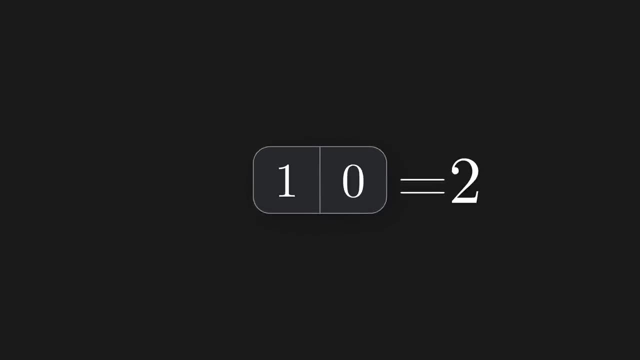 we can only do it for one state at a time. In this case, 7 squared, we get 49.. Quantum computers consist of qubits which also have two states: 0 or 1. But unlike a classical bit, a qubit doesn't have to be in just one state at a time. It can be in. 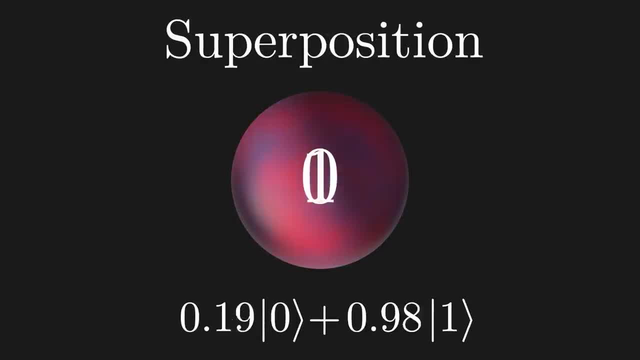 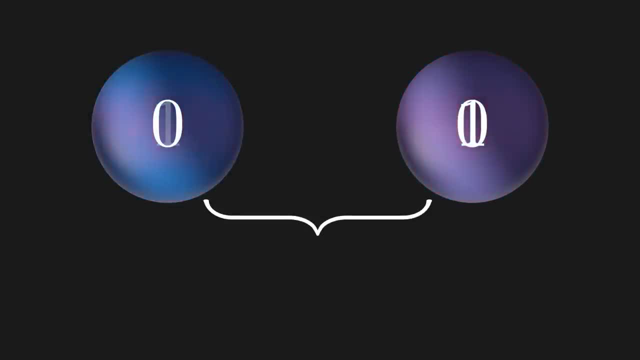 an arbitrary combination of those states, A superposition, if you will, of 0 and 1.. So if you have two qubits, they can exist simultaneously in a superposition of 0,, 1,, 2, and 3.. 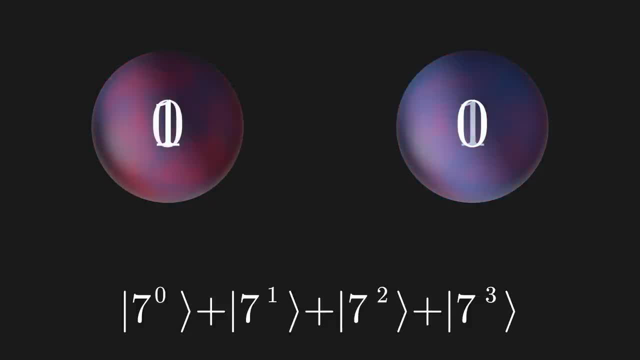 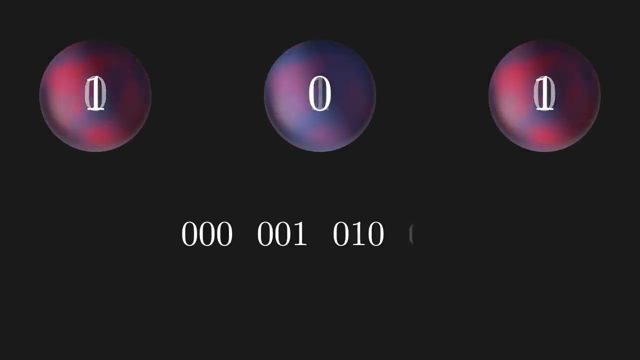 Now, when we repeat the same calculation, it will actually perform the calculation for all of those numbers at the same time, And what we're left with is a superposition of the different answers: 1,, 7,, 49, and 343.. If we add another qubit, we double the number. 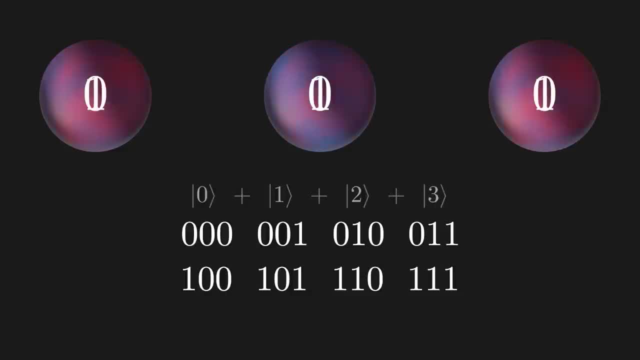 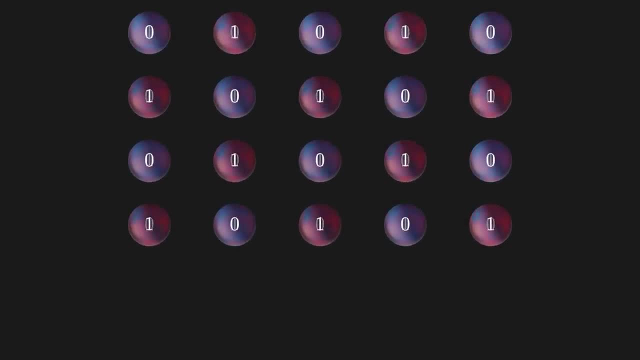 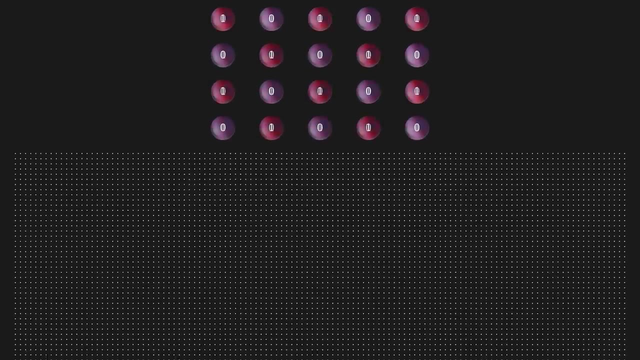 of possible states. So with 3 qubits we can represent 8 states and thus perform 8 calculations all at once. Increase that number to just 20 qubits and you can already represent over a million different states, Meaning you can simultaneously compute over a million different. 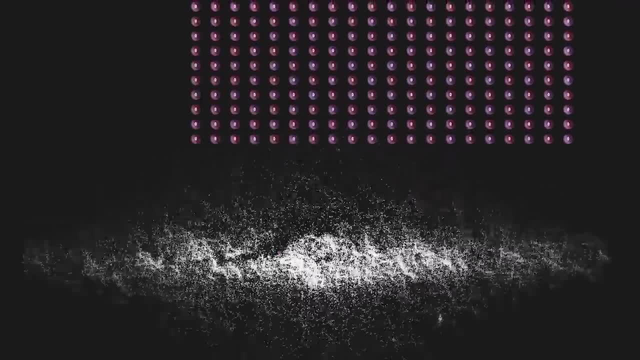 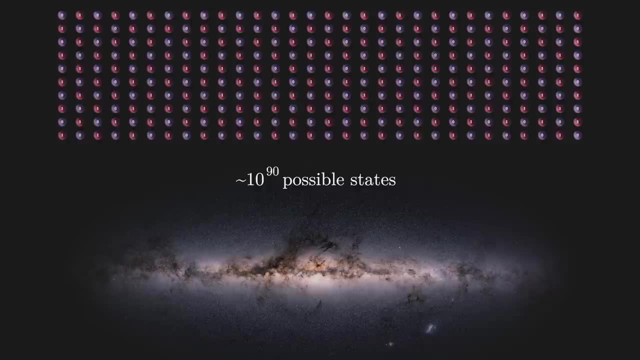 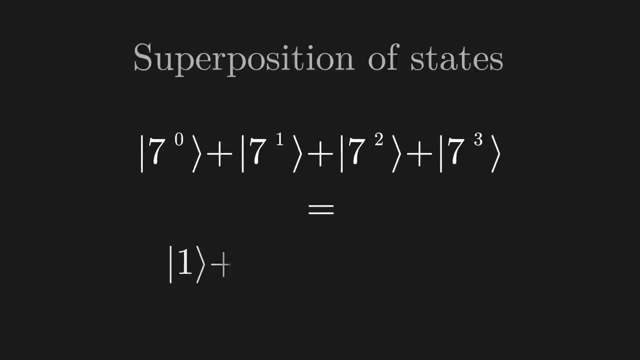 answers. With 300 qubits, you can represent more states than there are particles in the observable universe. This sounds incredibly powerful, and it is, But there is one very big catch: All of the answers to the computation are embedded in a superposition of states. 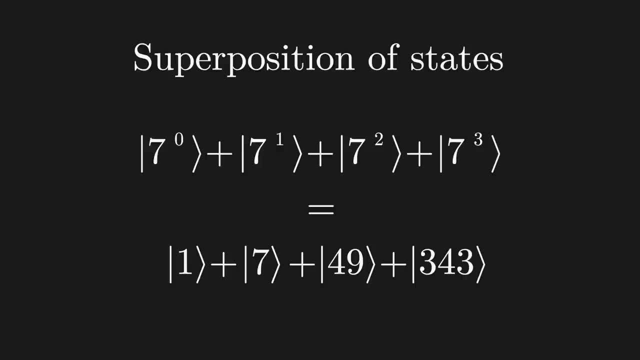 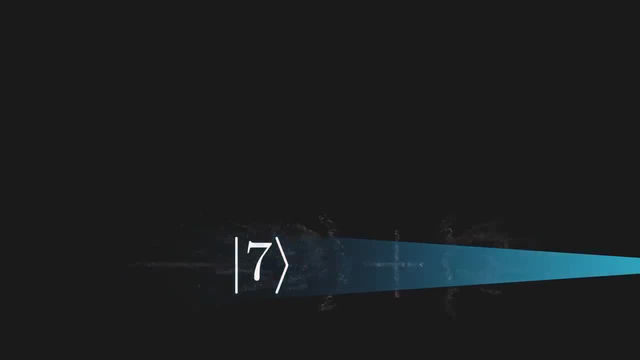 But you can't simply read out this superposition. When you make a measurement, you only get a single value from the superposition, basically at random, and all the other information is lost. So, in order to harness the power of a quantum computer, 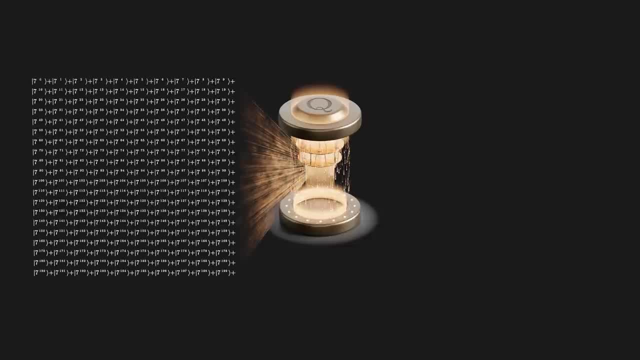 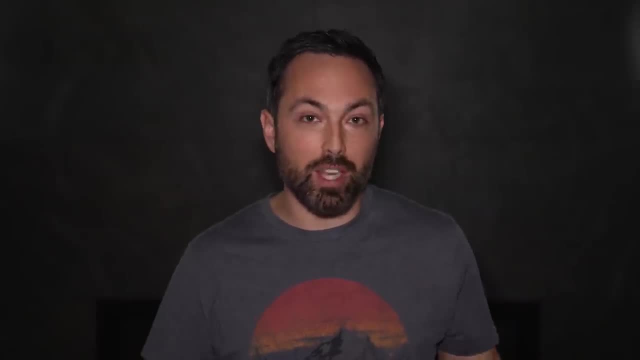 you need a smart way to convert a superposition of states into one that contains only the information you want. This is an incredibly difficult task, which is why, for most applications, quantum computers are useless. So far, we've only identified a few problems where we can actually 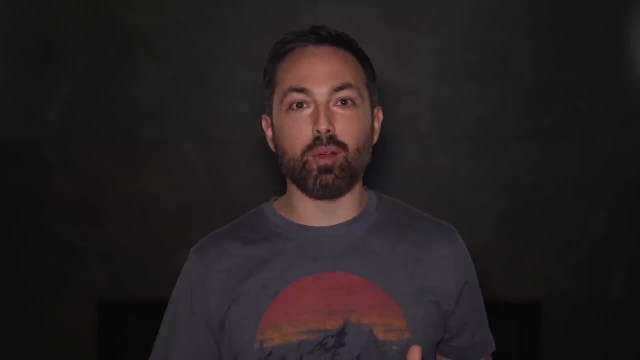 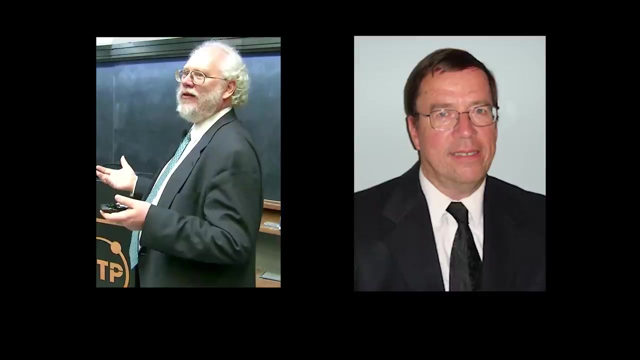 do this, But, as luck would have it, these are precisely the kind of problems that are the foundation of nearly all the public key cryptography we use today. In 1994, Peter Shore and Don Coppersmith figured out how to take a quantum Fourier transform. 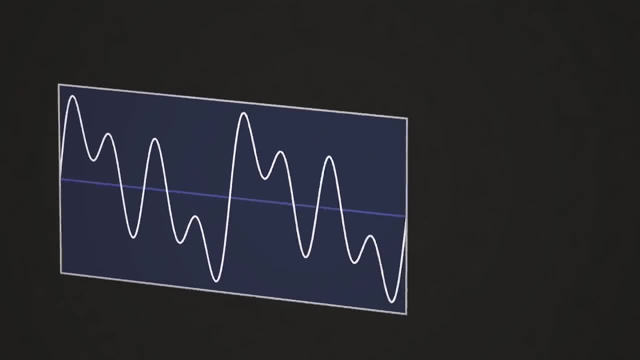 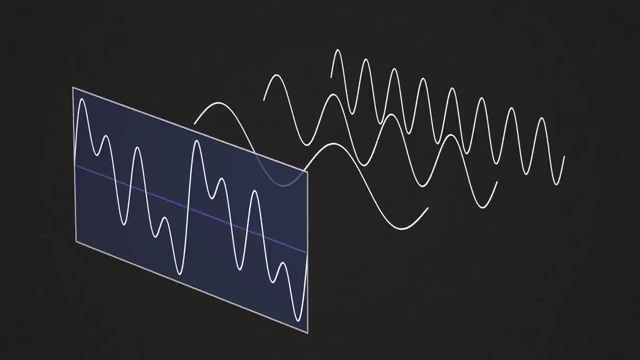 It works just like a normal Fourier transform. Apply it to some periodic signal and it returns the frequencies that are in that signal. Now this may not seem particularly interesting, but consider this: If we have a superposition of states that is periodic, that is the terms in the superposition. 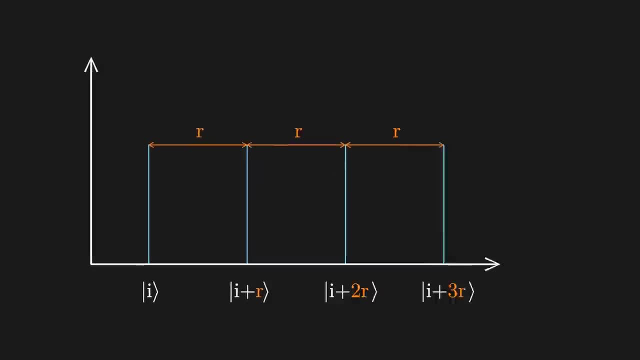 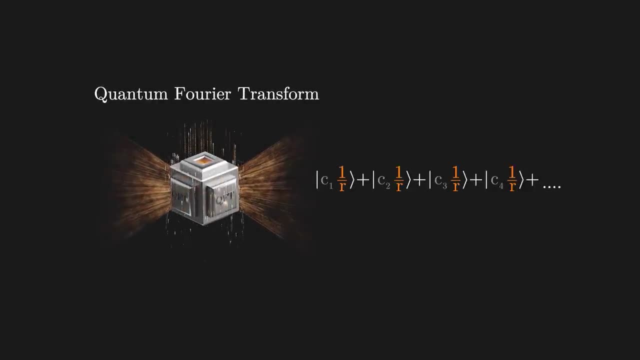 are separated by one, then we have a quantum Fourier transform. If we have a quantum Fourier transform, we can apply the quantum Fourier transform and we'll be left with states that contain the frequency of the signal. So this we can measure. The quantum Fourier transform allows. 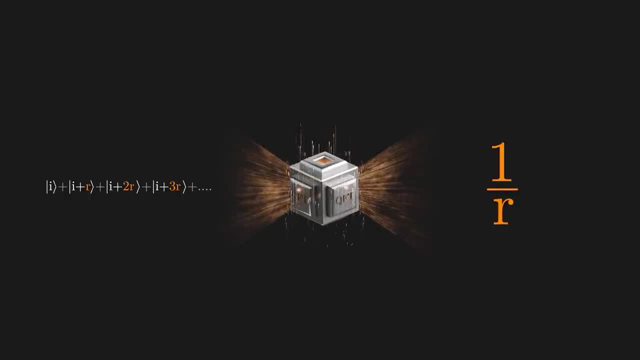 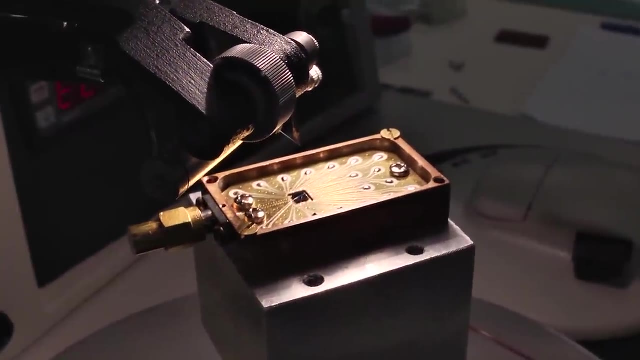 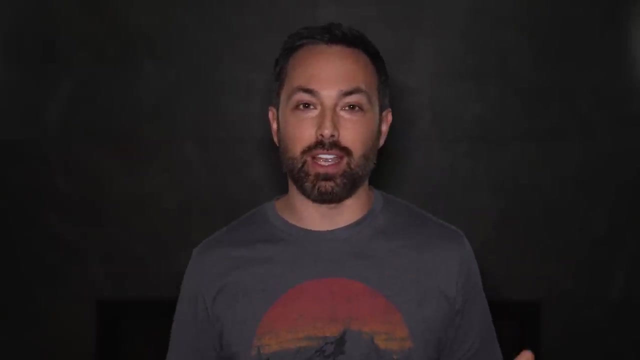 us to extract frequency information from a periodic superposition, and that is going to come in handy. So how does a quantum computer factor, the product of two primes, much faster than a conventional computer? I want to explain this by first walking through a simple example. 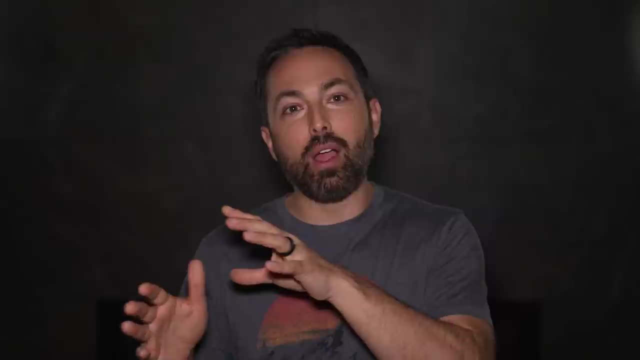 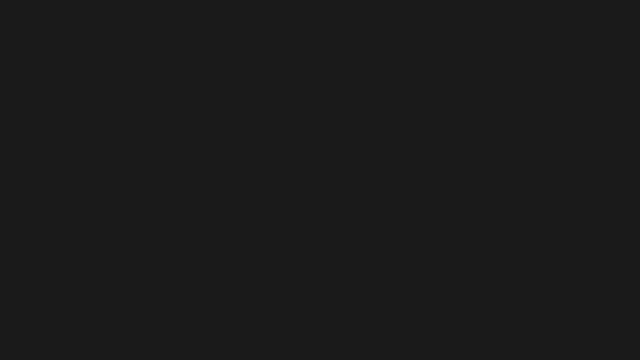 with no quantum computer required, and then I'll show how a quantum computer could execute this method, even for a very large number, in a short period of time. So let's say we have a number, n, which is the product of two primes, p and q. For the sake of this example, let's set n equal to 77.. 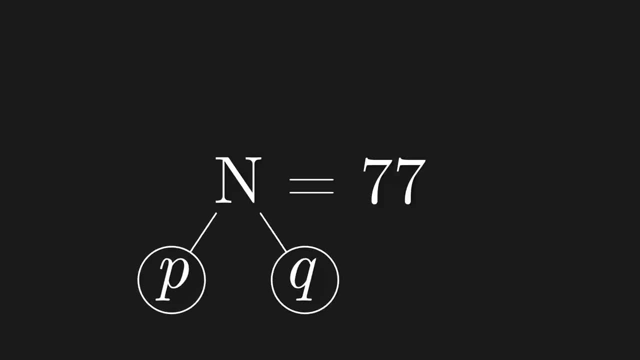 Now I bet you can guess the prime factors, but let's pretend for the moment that we don't know them, because with a product of really big primes we wouldn't. Now I want to use a fact about numbers that feels like magic. Pick a number, g, that doesn't share any factors with n. 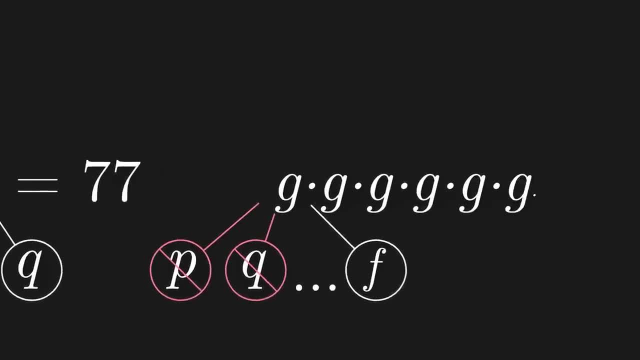 If you multiply g by itself over and over and over, you will always eventually reach a multiple of n plus one. In other words, you can always find some exponent r, such that g to the power of r is a multiple of n plus one. Let's see how this works. Pick any. 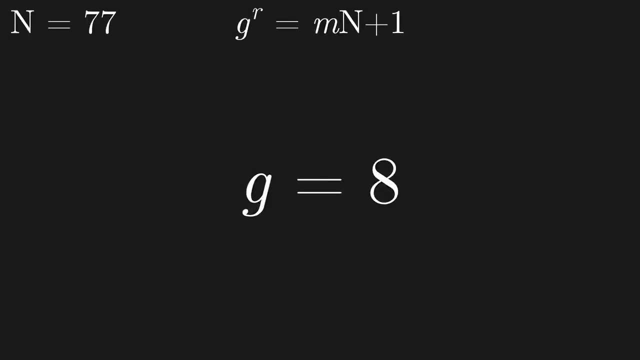 number that is smaller than 77. I'll pick the number eight. This number doesn't share factors with 77, and if you were doing this with big primes, it would also be extremely unlikely that you just happened to pick a number that shares factors with n. Now multiply eight by itself, once, twice, three times, four times. 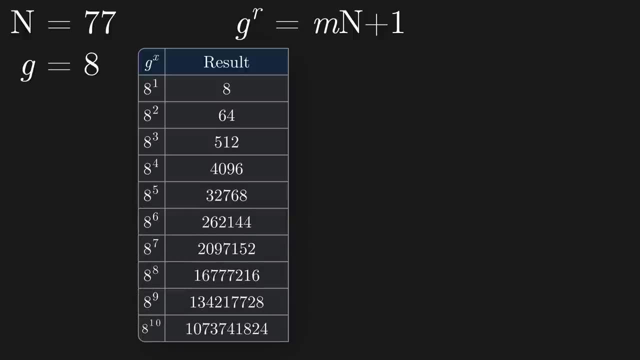 and so on, raising eight to ever higher powers, and then divide each of these numbers by 77. We're not really interested in how many times 77 goes into the number, just the remainder, what's left over. So let's say we have a number g, which is a multiple of n plus one. Let's say we have a. 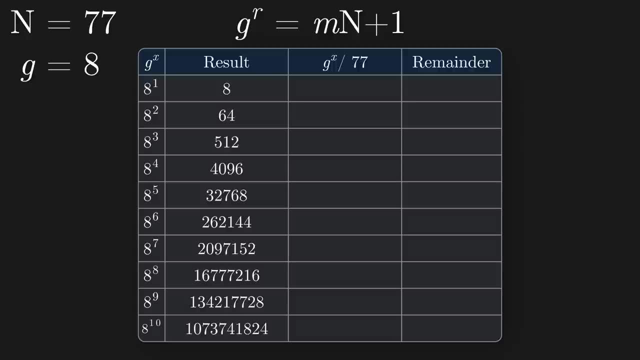 multiple of n plus four, because at some point 77 should divide one of these numbers with a remainder of exactly one. So eight divided by 77 is zero with a remainder of eight. Sixty-four divided by 77 is zero: remainder 64.. Five-twelve divided by 77 is six, remainder 50.. 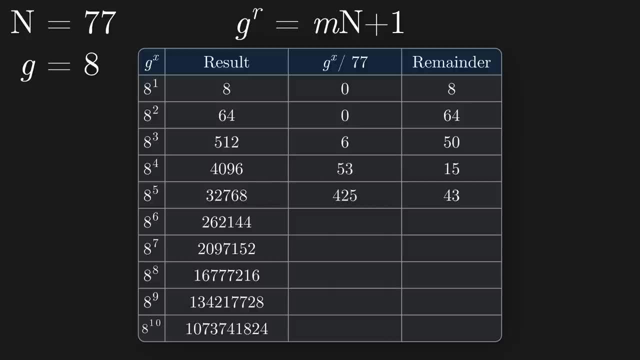 As we keep going, we get remainders of 15,, 43,, 36,, 57,, 71,, 29, and finally one, 1.. So there we have it. 8 to the power of 10 is one more than a multiple of 77.. 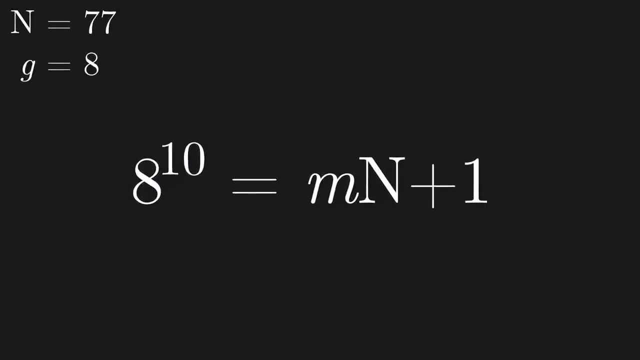 So we've found the exponent r, that satisfies this equation. But how does this help find the factors of n? Well, we rearrange the equation to bring 1 over to the left hand side, and then we can split it into two terms like so: And now, as long as r is even, we have 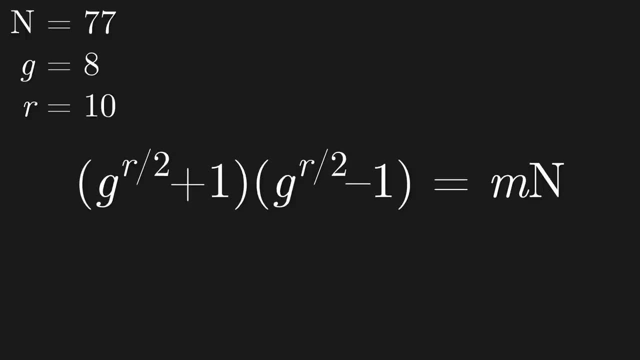 one integer times another integer is equal to a multiple of n. This looks remarkably similar to p times q equals n. I mean, since we know that p and q are on the right hand side of this equation, they must also be on the left hand side, just multiplied by some. 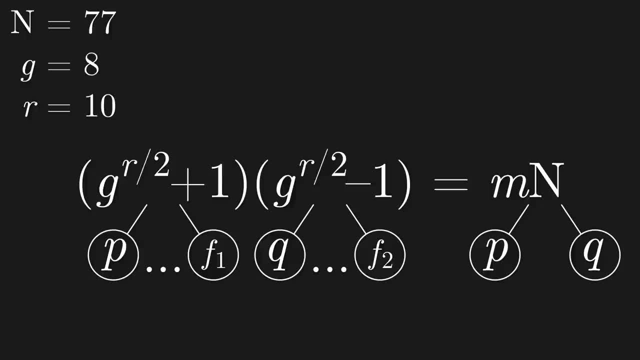 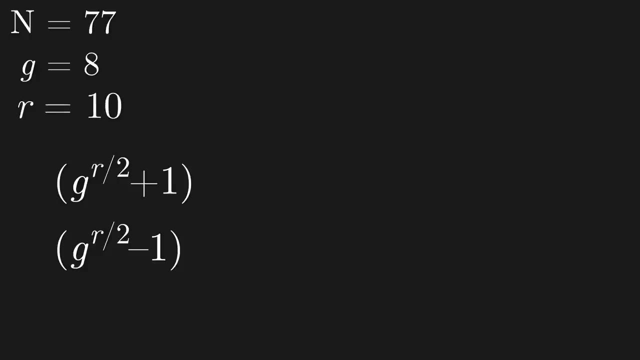 additional factors. So one way to think about what we've done is we've taken a bad guess for one of the factors g, and by finding the exponent r we've turned it into two much better guesses that probably do share factors with n. Since r was 10, the two terms 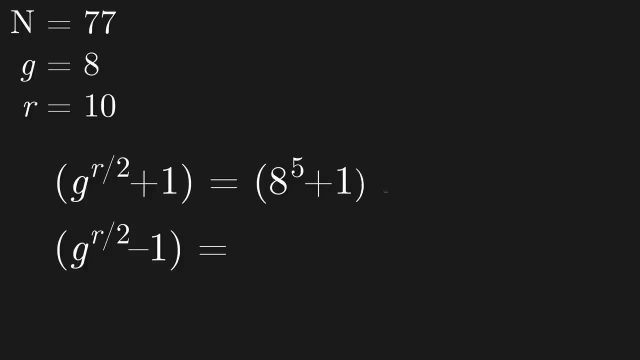 on the left hand side are 8 to the power of 5 plus 1, 32,769, and 8 to the power of 5 minus 1, 32,767.. These two numbers probably share factors with n, So how do we find them? 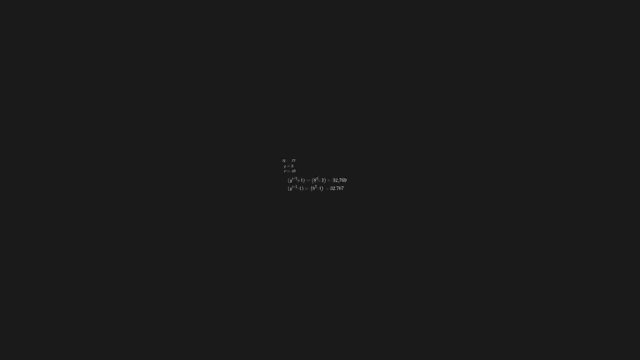 We use Euclid's Algorithm. Euclid's Algorithm: If you want to find the greatest common divisor of two numbers, say 32,769 and 77, divide the bigger number by the smaller one and record the remainder. In this case, 32,769 divided by 77 gives a remainder of. 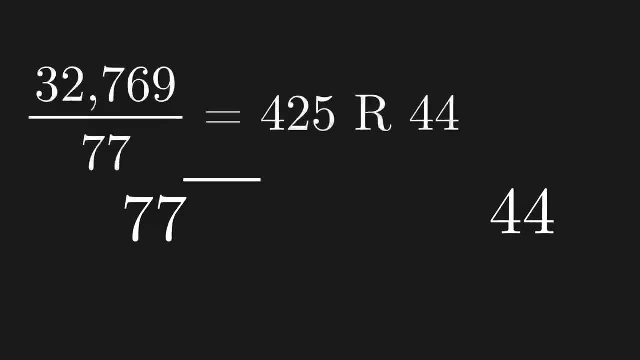 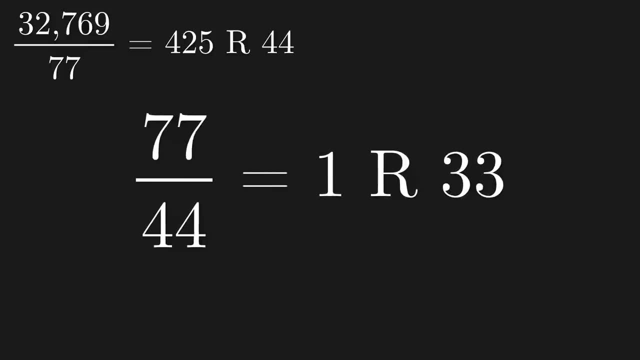 44. Then shift the numbers one position left and repeat. So now we divide 77 by 44, and we get a remainder of 33.. Repeat the process again: 44 divided by 33 gives a remainder of 11.. 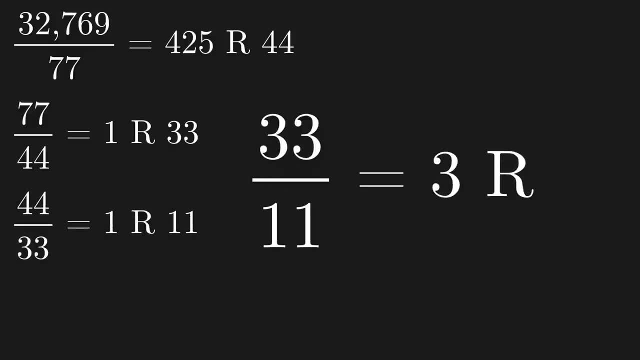 And again, 33 divided by 11 equals 3, remainder 0.. When the remainder is 0,, the divisor is the greatest common factor between the two numbers you started with- In this case it's 11, which is indeed a factor of 77 and 32,769.. You could do the same procedure with the other. 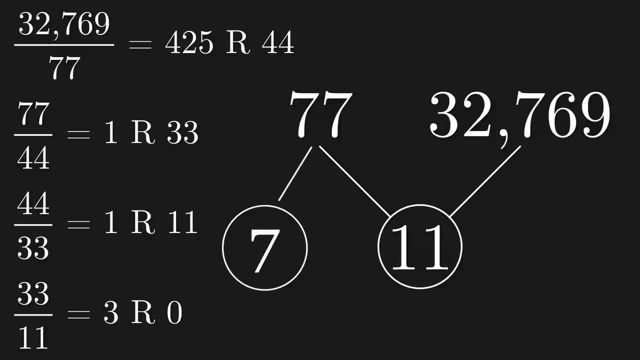 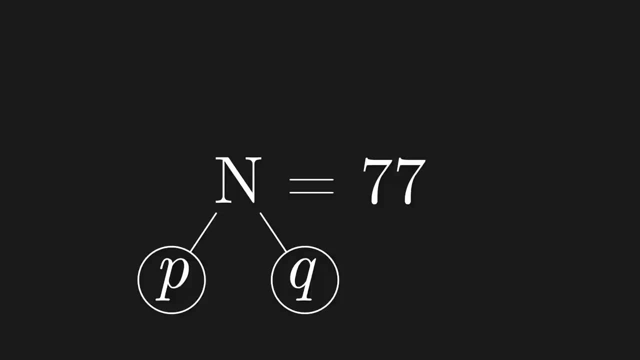 number. or just divide 77 by 11 to get 7,, its other prime factor. So to recap, if you want to find the prime factors p and q of a number, n first, make a bad guess, g Second. 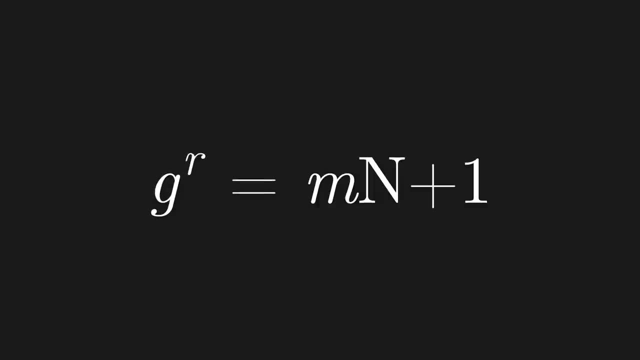 find out how many times r you have to multiply g by itself to reach one more than a multiple of n. Third, use that exponent to calculate two new numbers that probably do share factors with n. And finally, use Euclid's Algorithm to find the shared factors between those numbers. 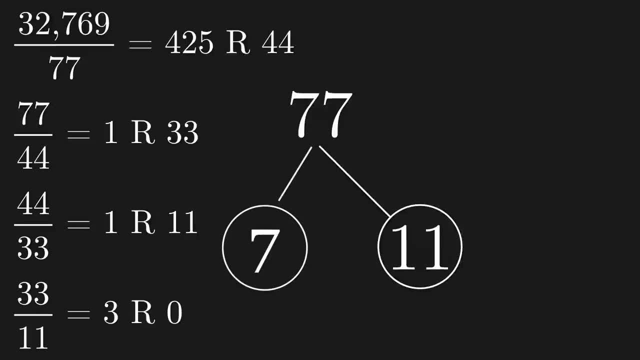 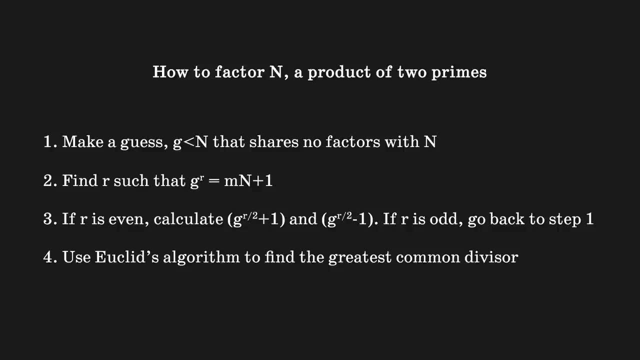 and n, which should give you p and q, Euclid's Algorithm. Now you don't need a quantum computer to run any of these steps, but on a classical computer this method wouldn't be any faster than other methods. The key process that a quantum computer speeds up is step two: finding. 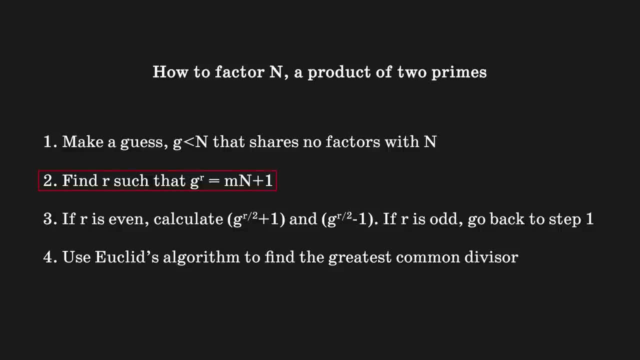 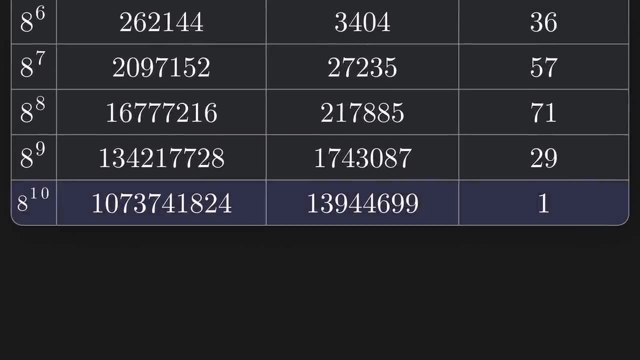 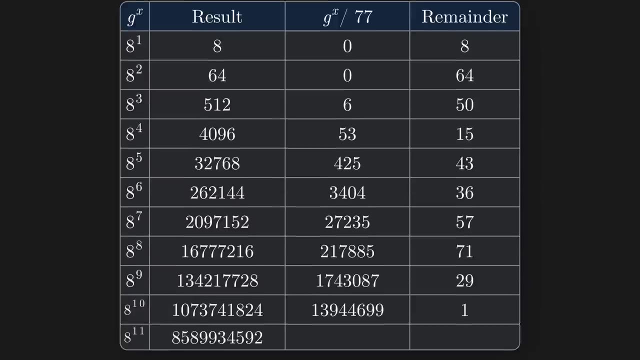 the exponent you raised g to to equal one more than a multiple of n. To see why, let's go back to our example where 8 to the power of 10 is one more than a multiple of 77. Watch what happens to the remainders if we keep going past 8 to the power of 10, to 8 to the. 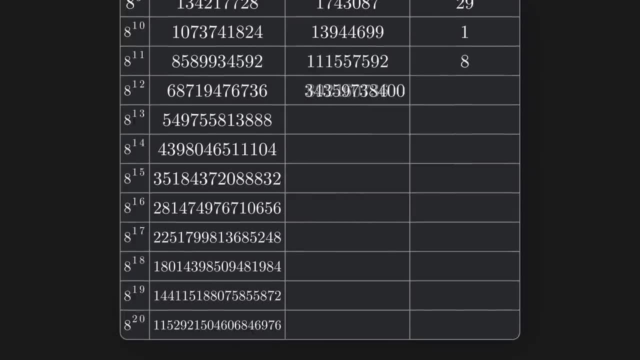 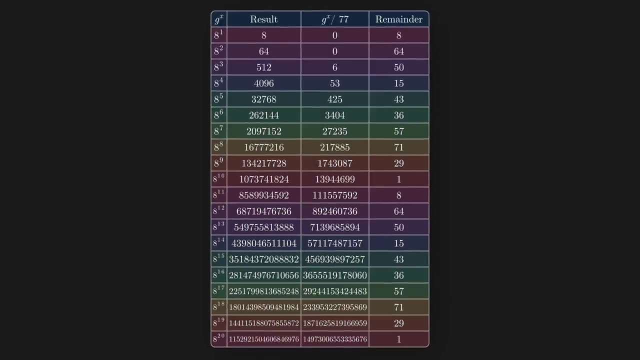 30,, 8 to the 24,, 9 to the 30…. Well, we get remainders of 8,, 64,, 50,, 15,, 43,, 36,, 57,, 71,, 29 and again…1!. The remainders SYCELL, and they will keep going. Notice how the exponent 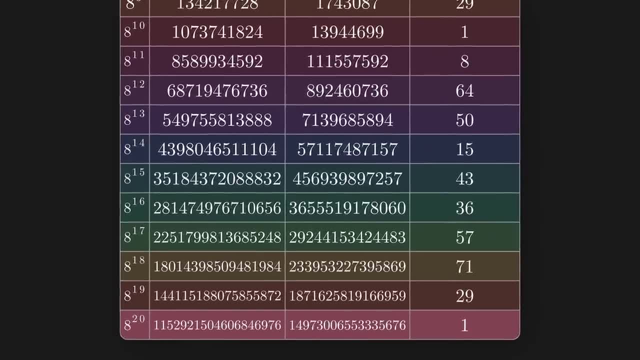 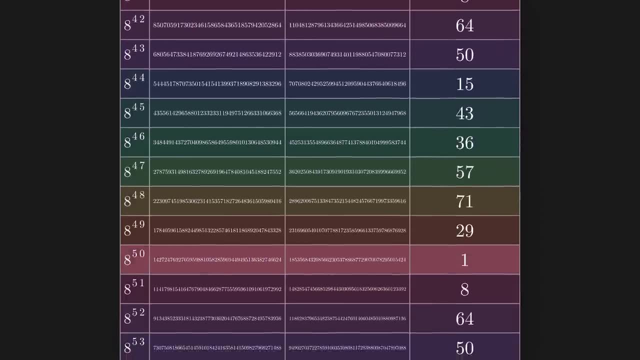 that yields 1 is 20,, which is 10 more than the first exponent yielded a remainder of 1.. 8 to the 30.. to the 48, raised to any power divisible by 10 will also be one more than a multiple of 77.. 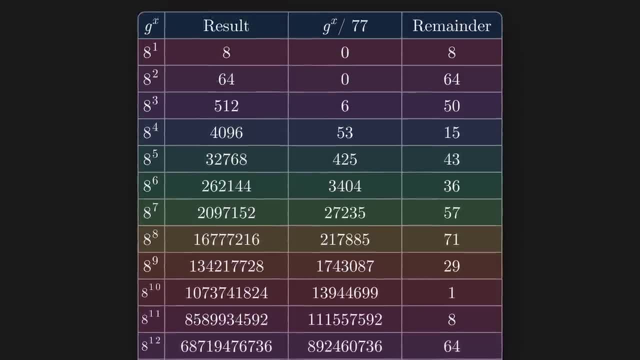 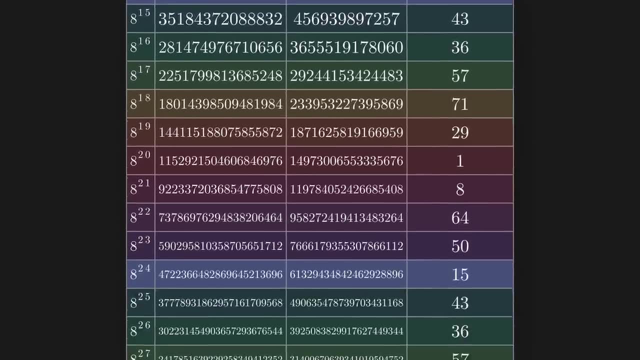 It's also worth noting that if you pick any remainder, say 15,, the next time you find that same remainder the exponent will have increased by 10.. So you can find the exponent R. that gets us to one more than a multiple of N. 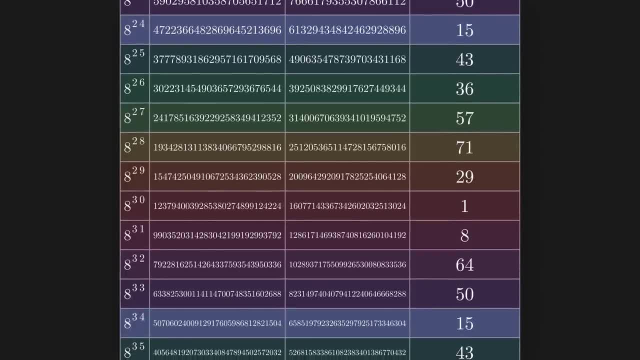 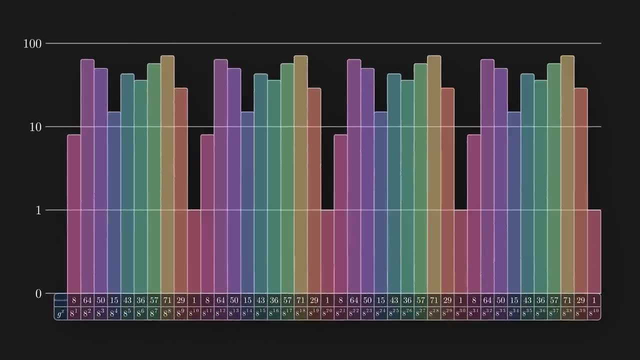 by looking at the spacing of any remainder, not just one. Remember that Here I'm plotting out the remainders on a log scale, so you can see they are periodic with a period of 10.. If I had made a different guess, 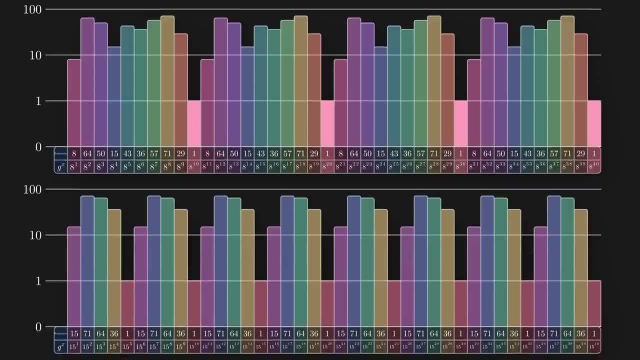 say I had picked, G equals 15 instead of eight. well then, the period would be different and the remainders would be different, but there would always be a remainder of one. Why is this? Well, now that you can see, this is a repeating pattern. 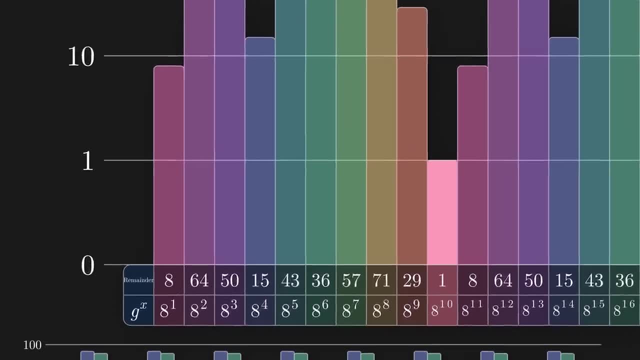 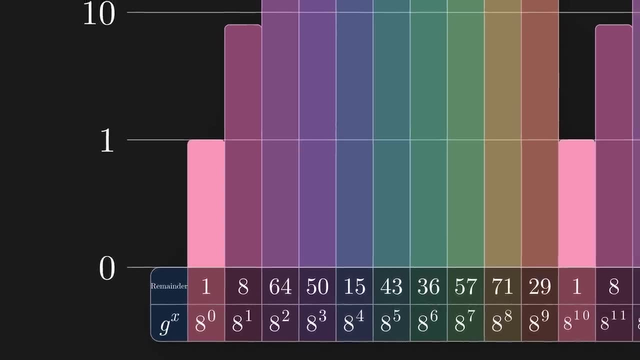 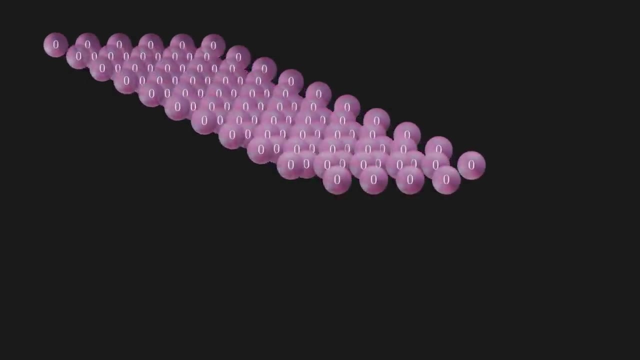 we can go back to the beginning, and any number raised to the power of zero is one. So that is actually the first remainder. So it must also appear when the cycle starts again. Now we are ready to use a quantum computer to factor any large product of two primes. 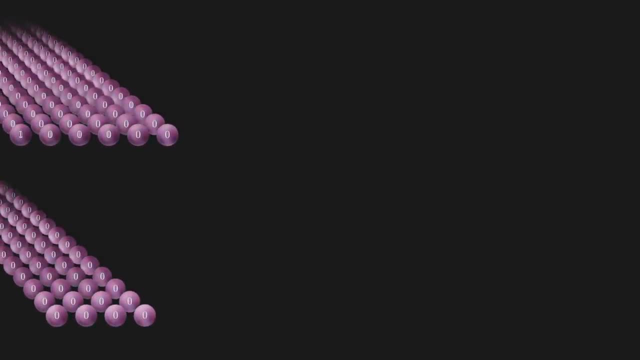 First we split up the qubits into two sets. The first set we prepare in a superposition of zero and one and two and three and four and five and six and seven and eight and nine, all the way up to 10, to the power of 1,234.. 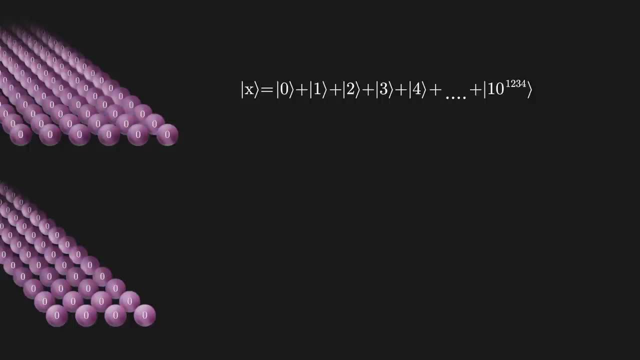 Yeah, This is a huge superposition, but if we had perfect qubits it would require only around 4,100.. The other set contains a similar number of qubits, all left in the zero state for now. Now we make our guess G. 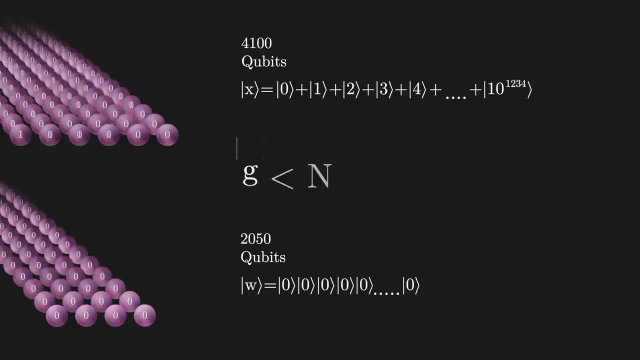 which most likely doesn't share factors with N. We raise G to the power of the first set of qubits and then we divide by N and store the remainder in the second set of qubits, leaving the first set of qubits as it was. 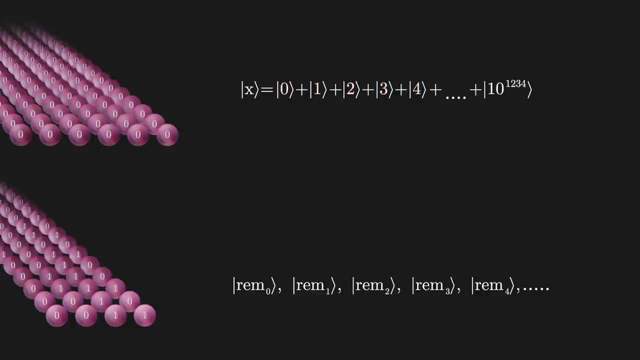 Now we have a superposition of all the numbers we started with and the remainder of raising G to the power of those numbers divided by N, And through this operation we have entangled our two sets of qubits. but we can't just measure this superposition. 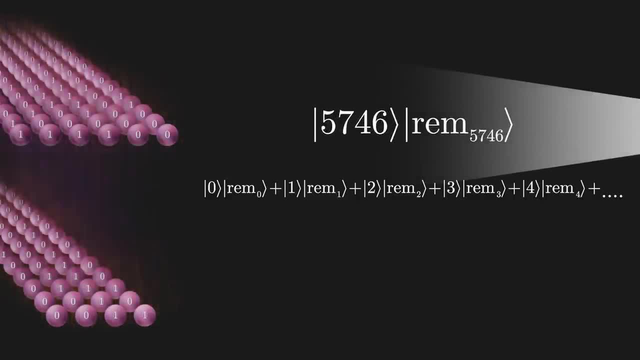 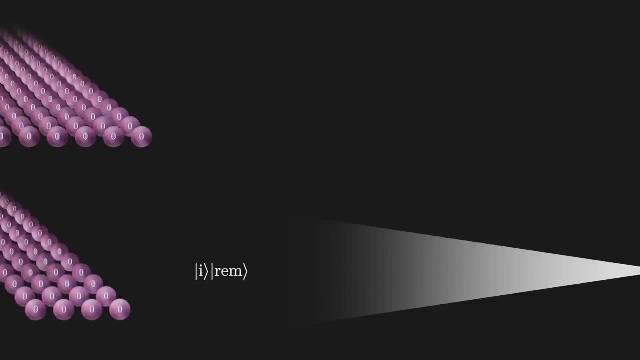 If we did, we would get a random value and learn nothing. But there is a trick we can use: If we don't measure the entire superposition, but only the remainder of the superposition, we will obtain some random remainder. But this remainder won't occur just once. 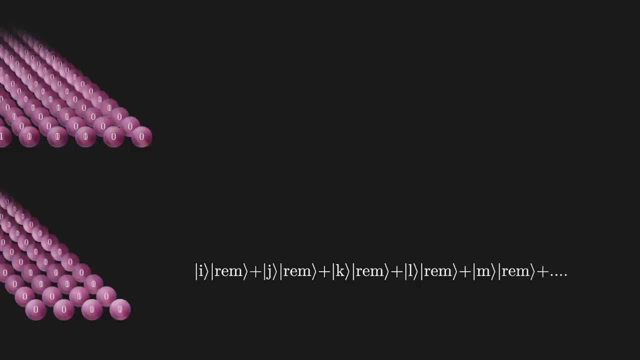 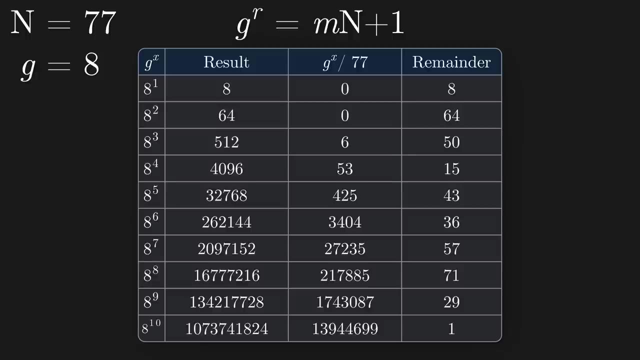 It will occur multiple times, every time it comes up in the cycle. Imagine we were doing this with the example from before, with N equals 77 and G equals eight. If the remainder we measured was, say, 15, then there would be multiple terms in our superposition. 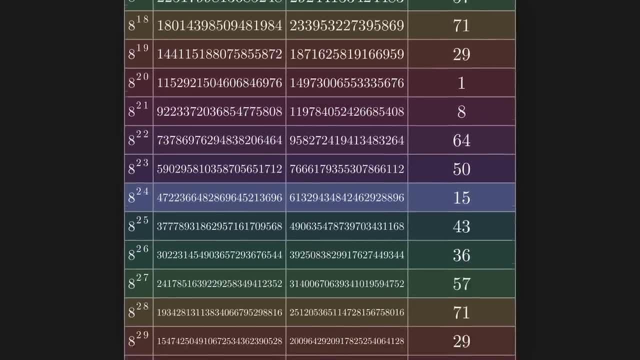 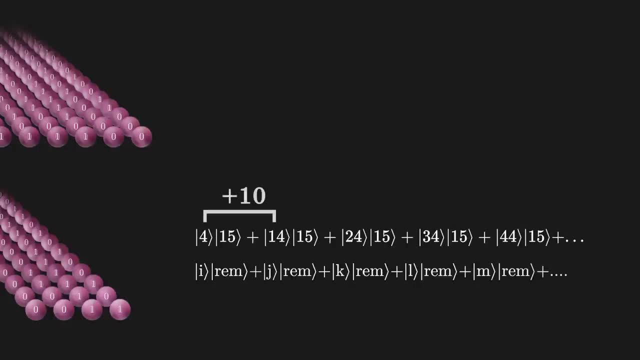 because there are multiple exponents. you can raise G to that. give this same remainder Exponents four, 14,, 24,, 34, and so on. They are each separated by 10. And that value is the exponent that satisfies our equation. 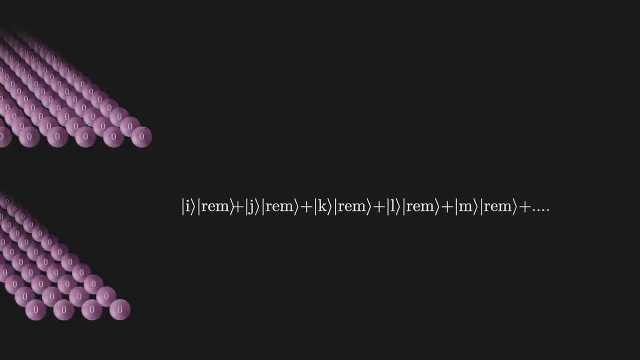 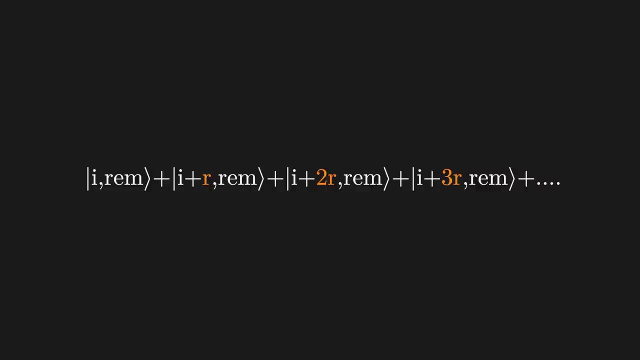 So, more generally, after measuring the remainder, we will be left with a superposition of states that all share the same remainder, And the exponents will all be separated by the same amount, R. This is the number we are looking for, Since the remainder is now the same for all states. 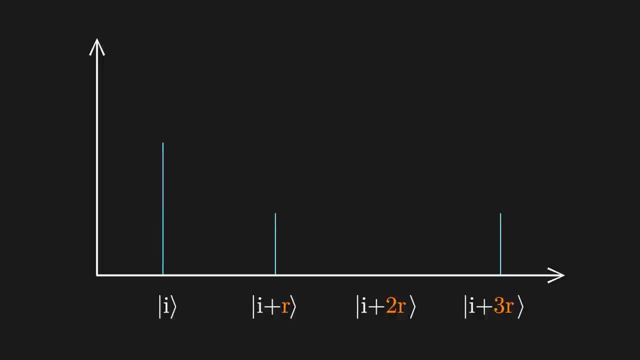 we can put it to the side And we now have a superposition that is periodic. Each term is separated from its neighbors by an amount R. If we now apply the quantum Fourier transform to this superposition of states, I'm simplifying a little here- 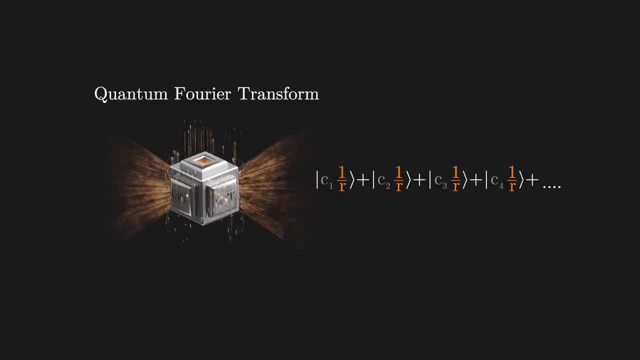 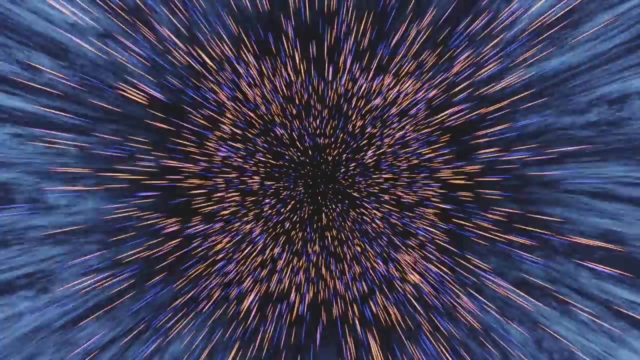 we will be left with states containing one over R. So all that's left to do now is perform a measurement and find R by inverting it, And that's it for the quantum part Now, as long as R turns out to be even. 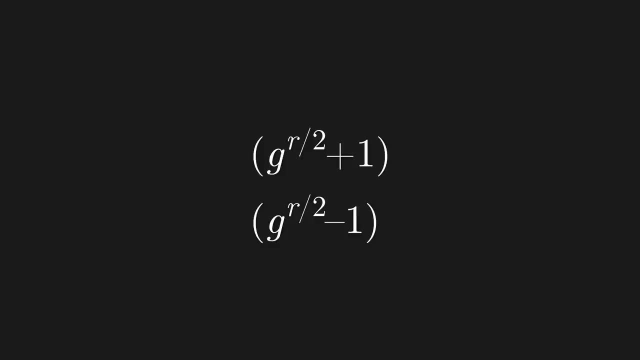 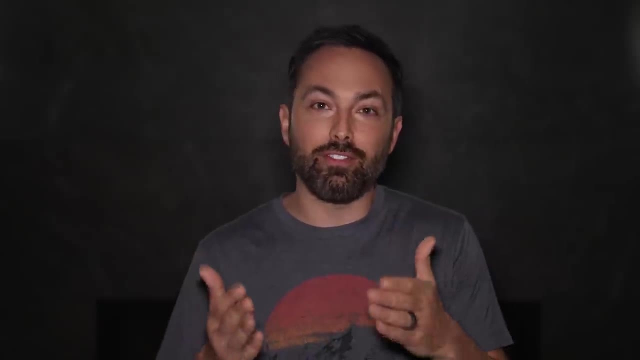 we can use R to turn our bad guess G into two numbers that likely share factors with N, And as long as these terms themselves are not a multiple of N, we can use Euclid's algorithm to find the factors of N and break the encryption. This would only take several thousand perfect qubits, but the qubits we have today are imperfect, So we need additional qubits to act as redundant information. In 2012,, it was estimated that it would take a billion physical qubits to break RSA encryption. 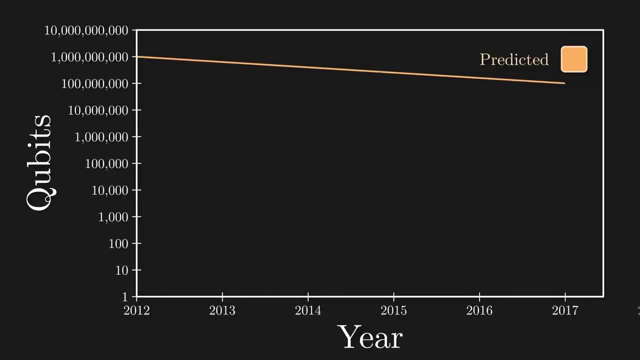 But by five years later, that number had dropped to 230 million, And in 2019, after more technological breakthroughs- that estimate plummeted to just 20 million physical qubits. So how many qubits do we have today? Well, if we look at the state of IBM's quantum computers. 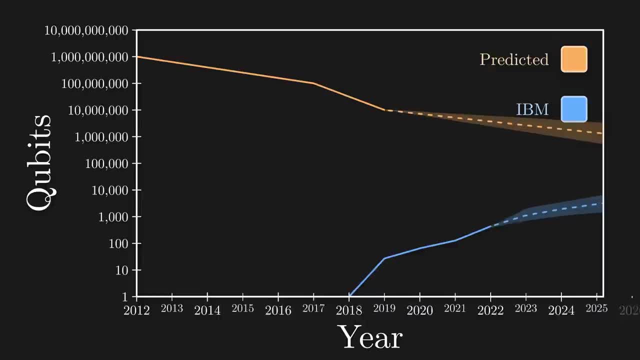 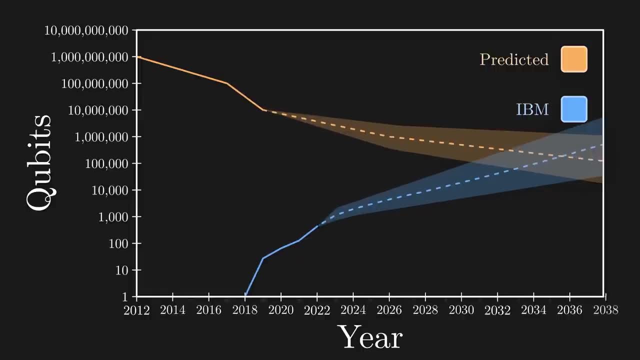 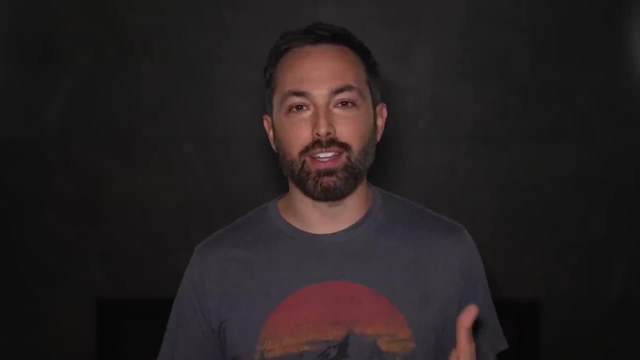 we are nowhere near that number of qubits, but progress looks to be exponential. So now it's just a question of when these two curves will collide before all our existing public computers, public key encryption can be broken, Because we've long known this threat is coming. 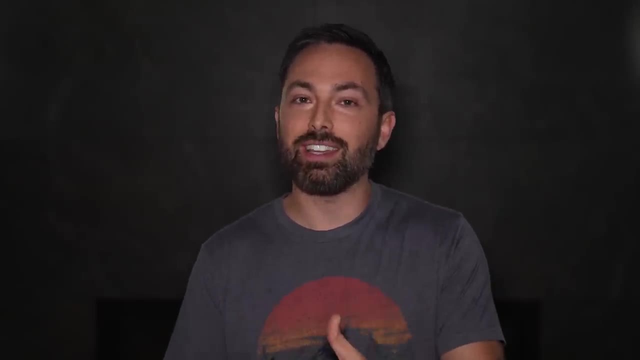 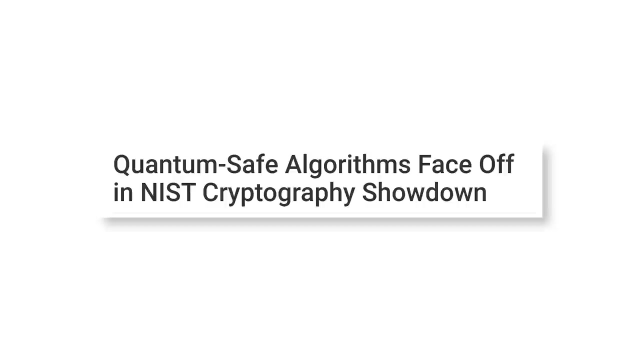 scientists have been looking for new ways to encrypt data which can withstand attacks from both normal and quantum computers. In 2016,, the National Institute of Standards and Technology, or NIST, launched a competition to find new encryption algorithms that aren't vulnerable to quantum computers. 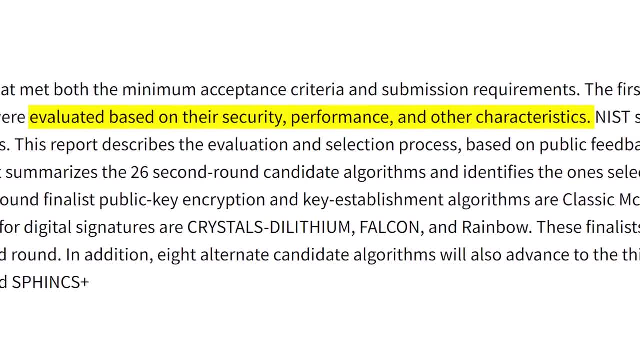 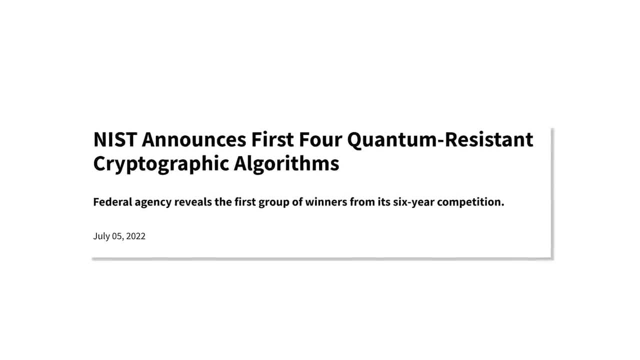 Cryptographers from all over the world submitted 82 different proposals, which were rigorously tested, some were broken, and then, on July 5th 2022, NIST selected four of the algorithms to be part of their post-quantum cryptographic standard. 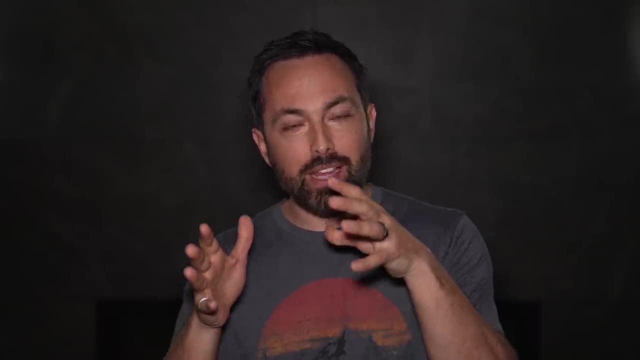 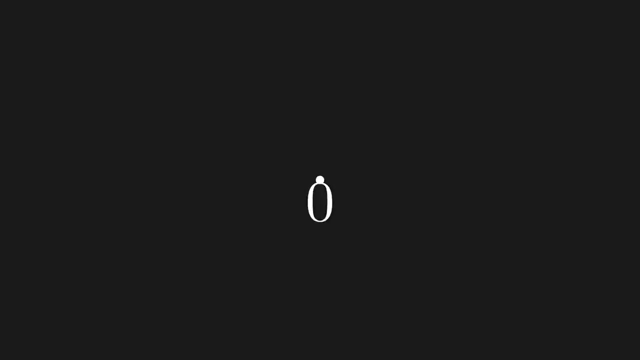 So how do they work? Well, three of the algorithms are based on the mathematics of lattices. So let's do a simple example. in the 2D plane, Take two vectors: R1 and R2.. By adding together different integer combinations, 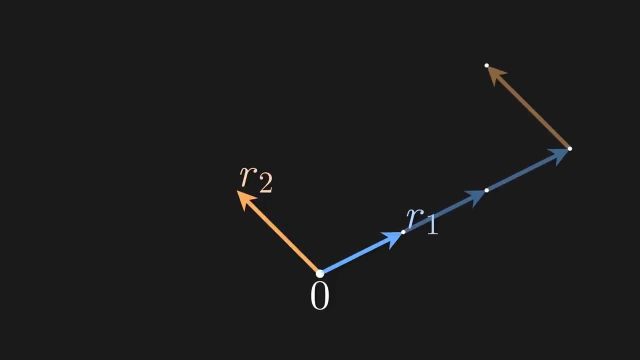 of these vectors, say three times R1 and one times R2, you can get two different points, And all the points give you two vectors. points you can get to by combining these two vectors in different ways is what is called a lattice. Now I will also give you the point C and your task is to tell me which combination. 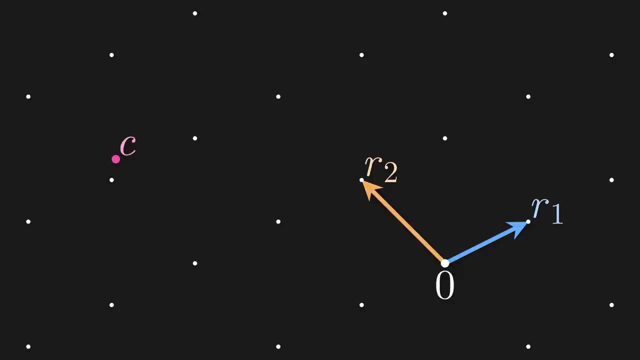 of R1 and R2 will bring me to the lattice point closest to C. It's pretty easy to see that we can get there by going in the direction of R2 twice and in the negative direction of R1 twice. Simple enough. But those vectors, R1 and R2, are not the only vectors that can. 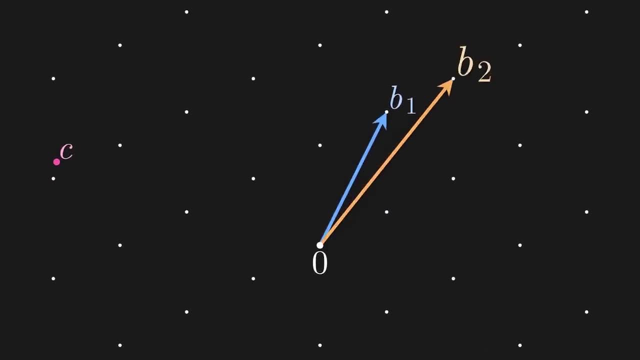 give you this lattice. Take B1 and B2, for example. These vectors also build up the same lattice. And now, if I ask you the same question again, can you tell me the combination of B1 and B2 that gets you to the lattice point closest to C? This has become a lot harder. 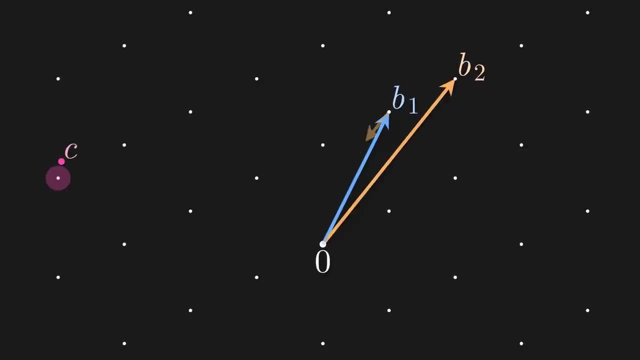 But why is that? Each time we're taking a step, we're trying to get closer in either the X or Y direction, But with the B vectors, each time we take a step in the right direction with one vector, it puts us off in the other direction, And that's why these vectors are a lot harder. 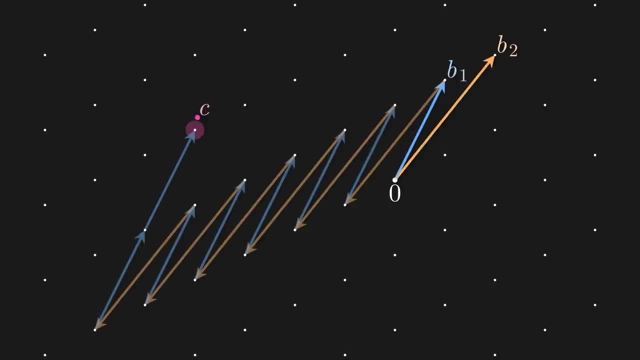 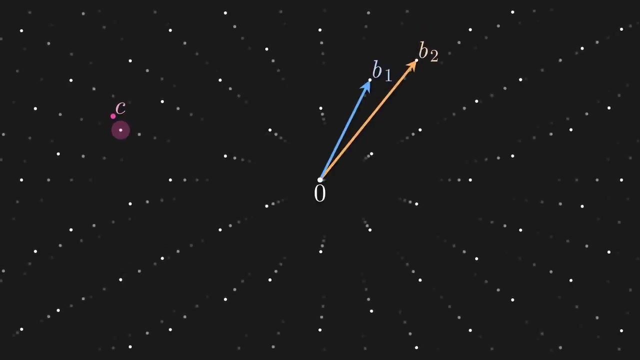 to work with. In the end it takes us a combination of 8 times B1 and negative 6 times B2 to get to the closest lattice point. That is a lot harder than before, but it's still a relatively easy problem to solve. But if we extend it to three dimensions, this already becomes 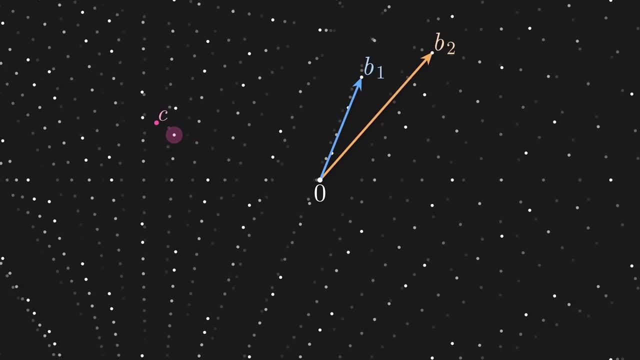 a lot harder, Especially because you're not given the collection of all lattice points. you're only given the vectors that make it up. So when you find a lattice point close to the target, you must still find all the other lattice points near it to make sure yours is indeed the closest. 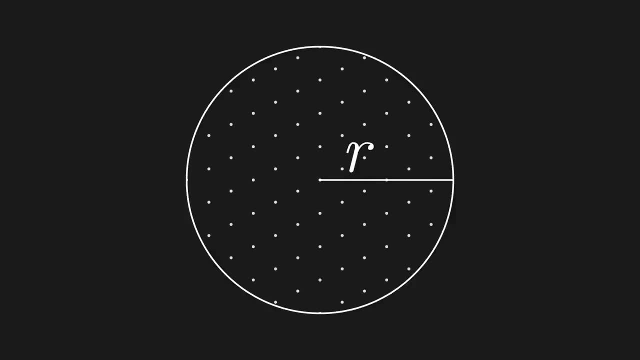 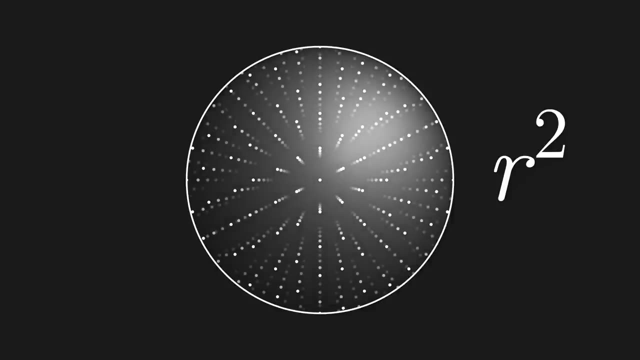 Let's take a circle of radius r in two dimensions, The number of lattice points inside the circle is proportional to r squared. Add a third dimension and the number of points in the sphere is proportional to r cubed. So just watch how the number of lattice points grows. 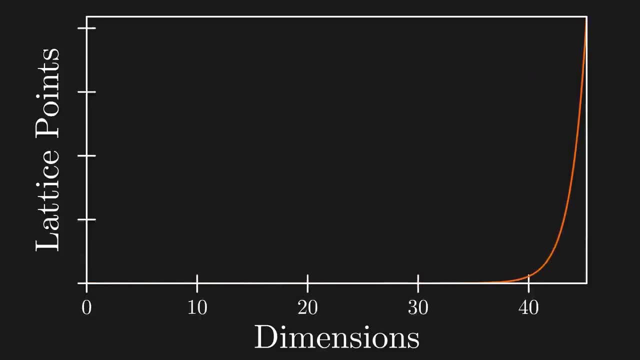 as we increase the number of dimensions. Solving the Closest Vector Problem. Solving the Closest Vector Problem. Solving the Closest Vector Problem problem is a piece of cake for your computer. in three dimensions, Even a hundred dimensions should be manageable. But in proposed future encryption. 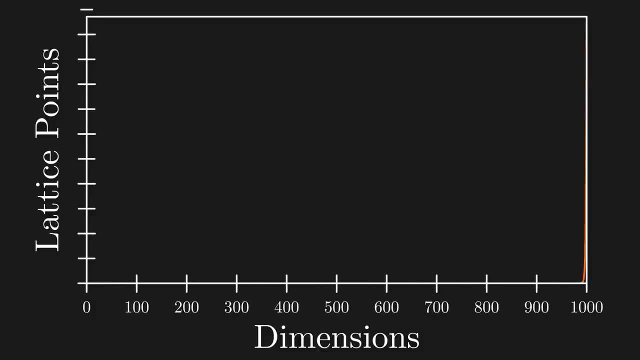 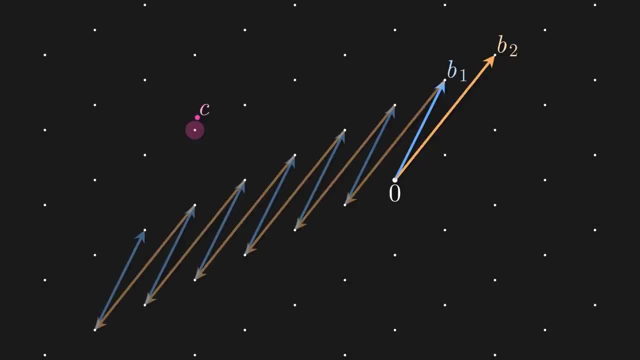 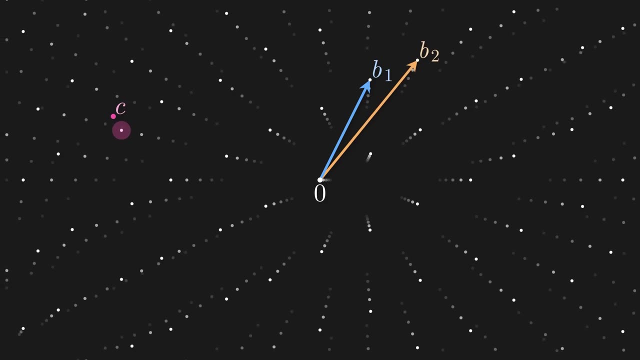 schemes, we'll use around a thousand dimensions. Take one step in the right direction on one of those dimensions and you could potentially be taking a wrong step in the other 999 dimensions. You win some, you lose everything else. With that many dimensions, it becomes extremely hard to find the closest point, even for 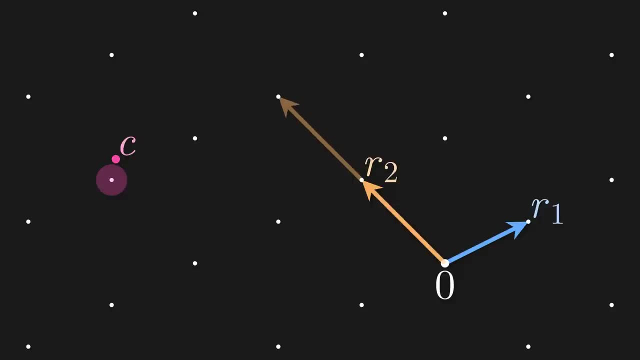 the most powerful computers, That is, unless you know a good set of vectors. So how do we use that to encrypt data? Well, let's go back to our two-dimensional example. Each person has a good set of vectors that describes a lattice, but 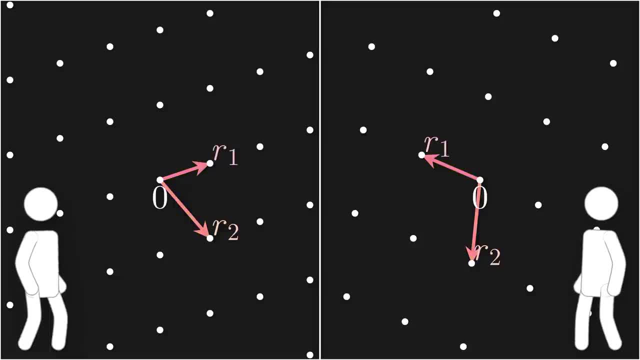 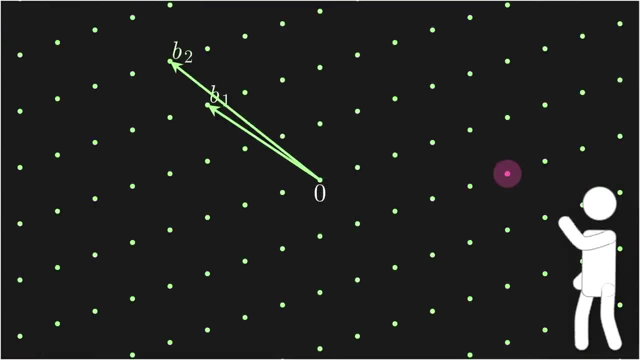 they keep these vectors secret and they only share their lattice publicly, using a set of vectors that is hard to work with. Now, if I want to send someone a message, I pick a point on their lattice. For example, say this point corresponds to the number. 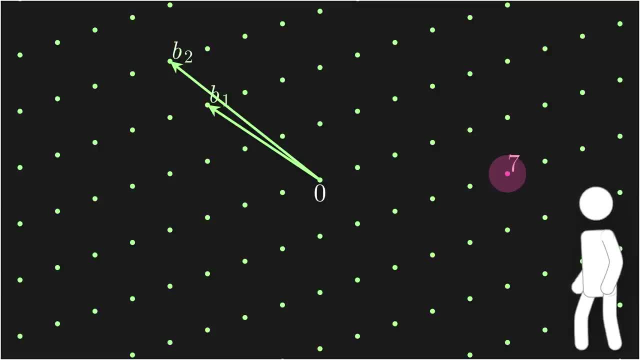 7.. So if I want to send the number 7, I can take that point but then add some random noise to it. So the message I send is not precisely at that point, but close to it. Now to decode the message, my recipient must figure out which lattice. 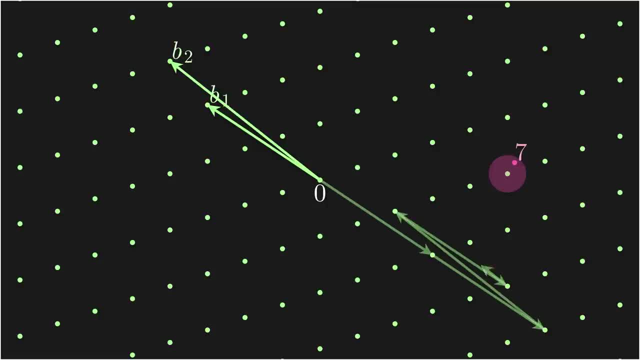 point is closest to the message point In a thousand dimensions. this will be extremely hard to do unless you have the nice set of vectors which my recipient does. So it's easy for the recipient who has the good vectors, but hard for everyone else And as far as we know this problem 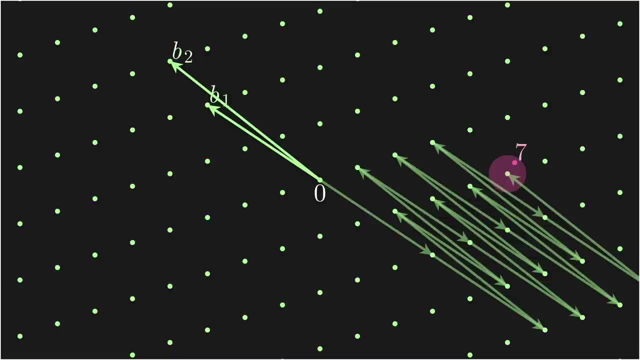 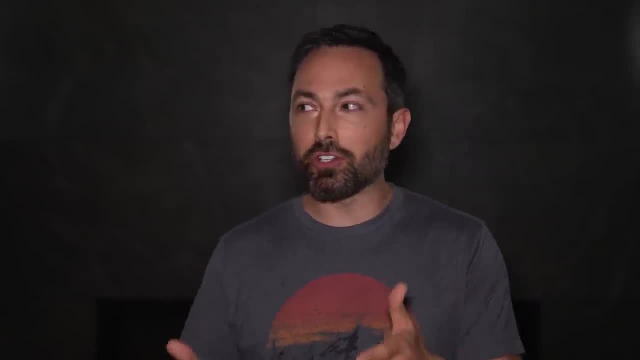 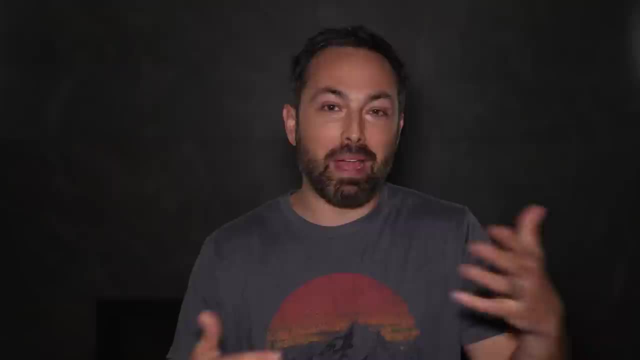 is extremely difficult to solve for both normal and quantum computers. Behind the scenes, there is an army of researchers, mathematicians and cryptographers working to make sure your secret data stays secret. These are some of the unsung heroes that will keep us safe, moving forward, avoiding mass surveillance. 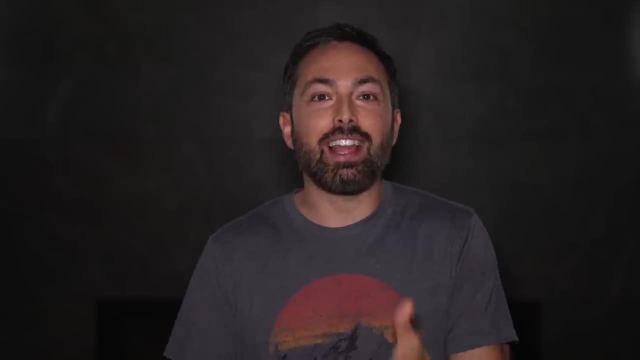 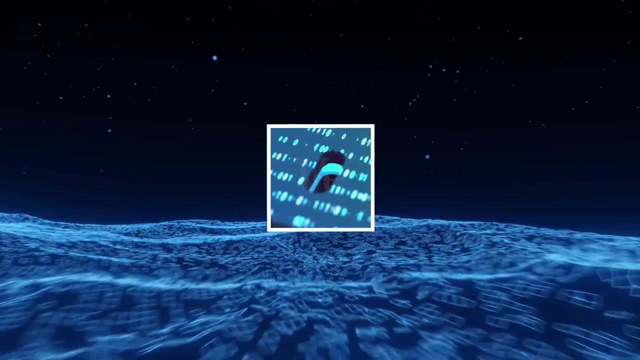 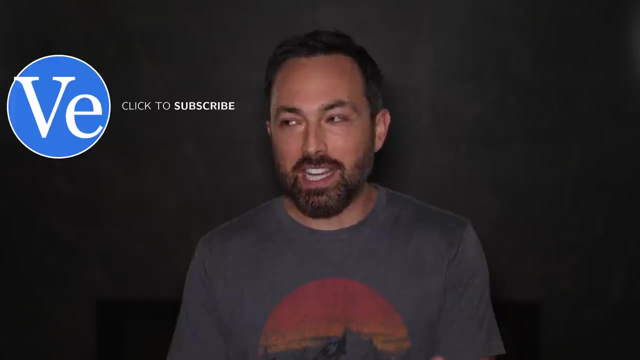 by governments keeping critical infrastructure protected and allowing you to live as if quantum computers were safe. Something that fascinates me is being able to see where the world is headed, And right now it's clear that quantum computers and AI chatbots are going to play bigger and bigger. 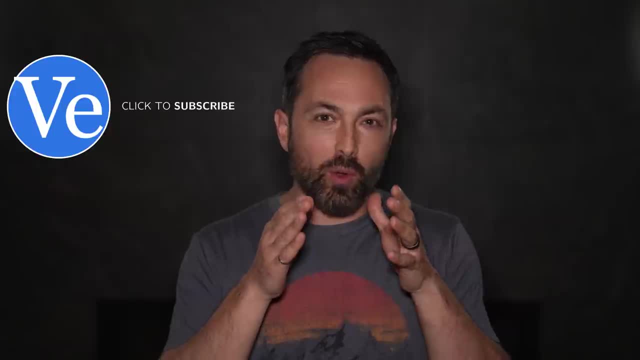 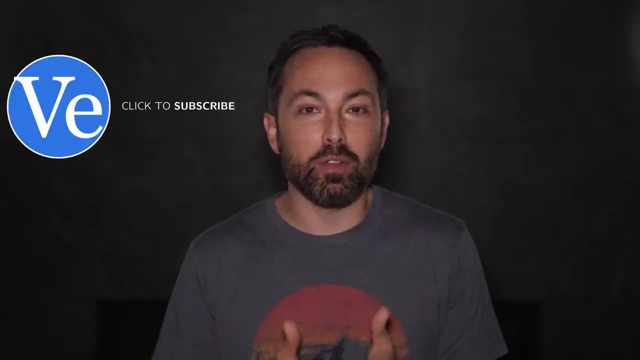 roles in our lives in the coming decades, Even if we don't know exactly how they'll be implemented. I think it's important to learn how they work right now, And you can do that with this video's sponsor, Brilliant. Brilliant has an incredible course on quantum algorithms. This one was co-developed.